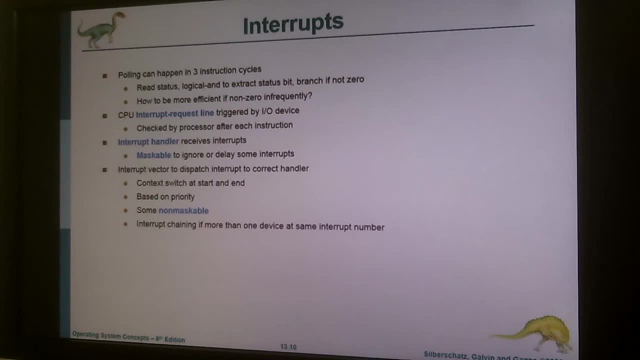 It's a really complicated system. The operating system itself is managing the memory, managing the CPU, managing the operating system itself. It processes itself. And what else you're managing? You're managing the IOS system, right? What else You manage? the ports, USB ports, whatever, HDMI ports, et cetera, et cetera. 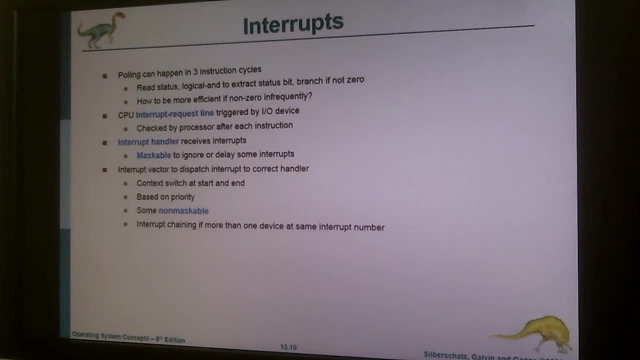 All those IOD devices are controlled by the operating system. Plus, since almost all of the operating systems are network operating systems right now, even your personal Windows computer is a multi-user network-enabled operating system. right, That means you have tons of stuff about security, data protection. That is a part of the operating system too. 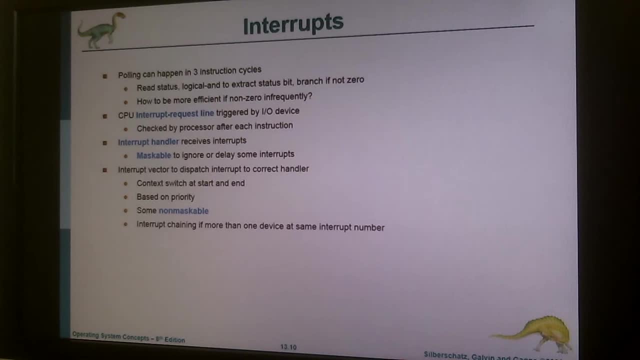 So it has to be complex. I mean that operating system has to be complex, All right, There are two types of interrupts. One is maskable, The other one is non-maskable. Maskable means you can change its priority or its place in the interrupt queue. You can change it. All right, As a user, your application can change it. 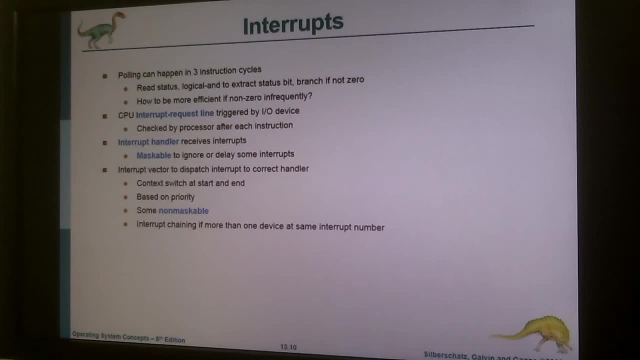 But there are interrupts that you cannot touch, which are non-maskable. All right, Those are. for what kind of processes do you think If you cannot mask an interrupt, if you cannot touch an interrupt, what kind of interrupt it could be? What kind of process should be assigned to this interrupt? 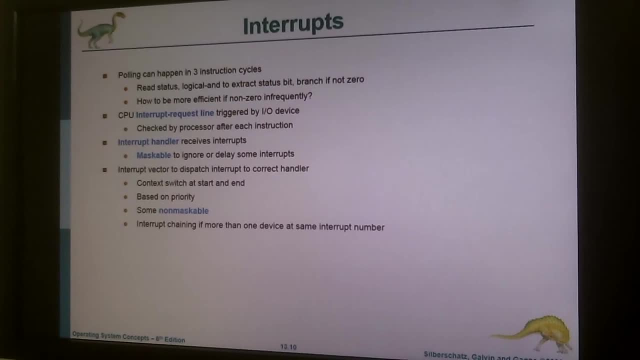 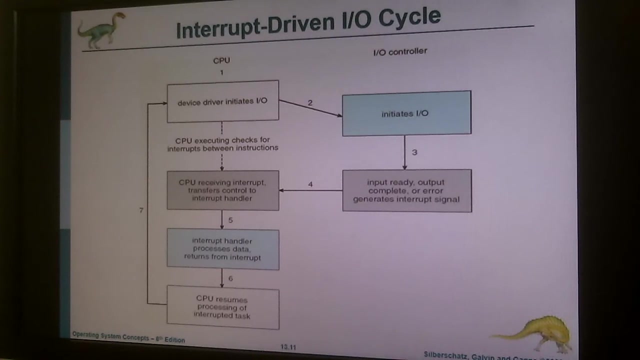 Core programs? I guess Yes. core programs meaning kernel mode, system calls and things like that. right, The operating system, core applications Like memory management, Like CPU management, interrupts. There is a diagram here talking about how can you handle an IO device roughly. Basically it's saying that you know in the CPU you're running a process and that process needs to do an IO request. 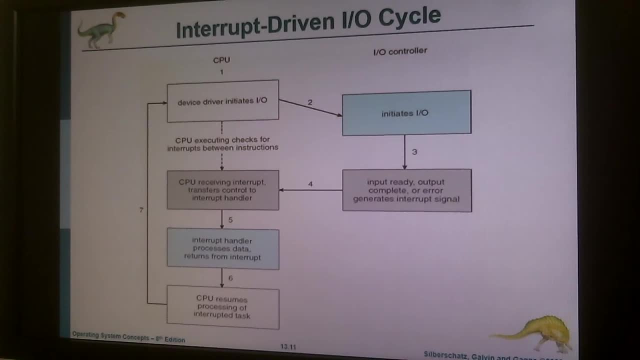 In that case you just generate an interrupt, tell the CPU that I need to go to an you know, talk to my IO device And save the state of the PCB, save it in the queue and then do something else in the meantime. 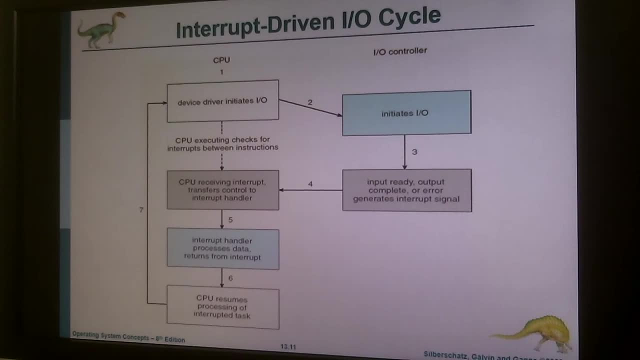 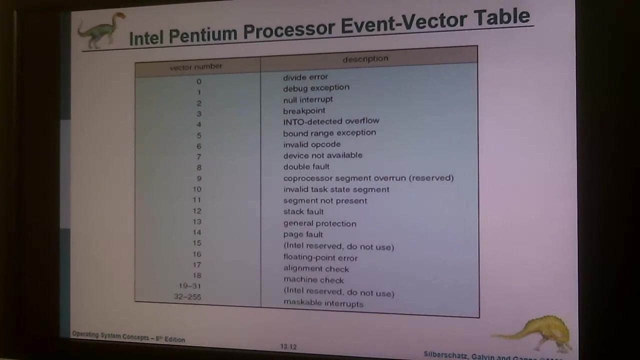 After all, your interrupt will tell you that I'm done with the IO And your CPU will reload that process and do whatever it's supposed to do with the new data and finish it up and done for the next job. And interrupts are saved in a list. 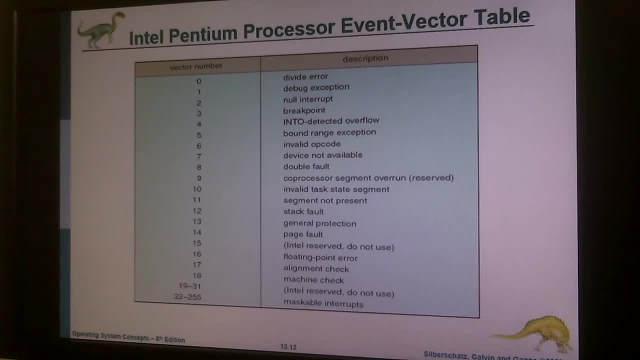 As I was saying before, in a table. That table is called vector table And the process and the interrupt number is actually matched, And some of the interrupts are non-maskable, as I said, which means you cannot touch. Those are system interrupts. Let's call it system interrupts, right. 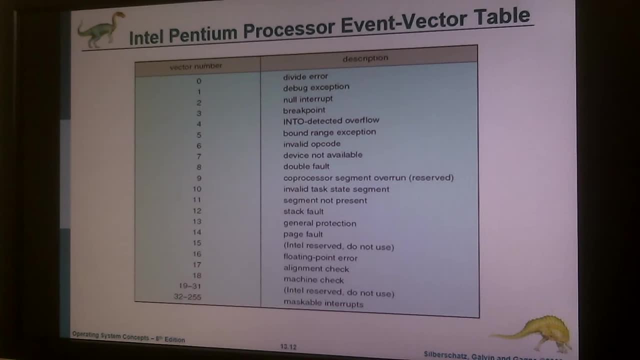 And an example for that: on the screen says: divide- error 0. Divide by 0- error. for example, Interrupt 0.. You can never change its priority and you can never change its place in the queue. You can't do that. 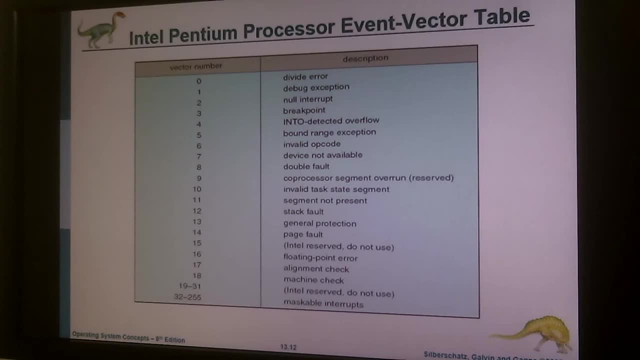 Because it's very important system-wise, right For example, another one, another super important one is page fault, number 14.. Page fault is also virtual memory management, right Page management. So it is very important if you touch that as a user, if your application changes anything in the system stack. 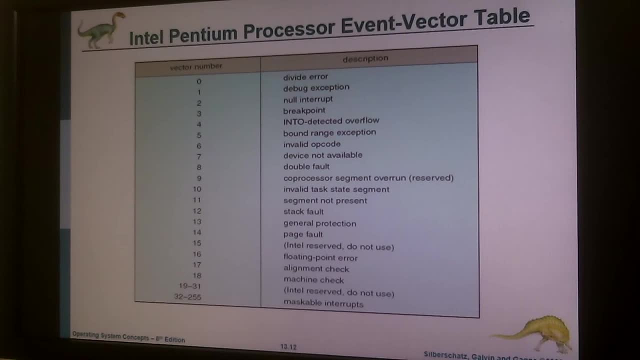 system data structures, it will be a problem: Floating point errors, et cetera, et cetera. And after 32,, after 255, it's your interrupt stuff. I mean, if you write an application, your application uses any interrupt numbers between 32 and 255. 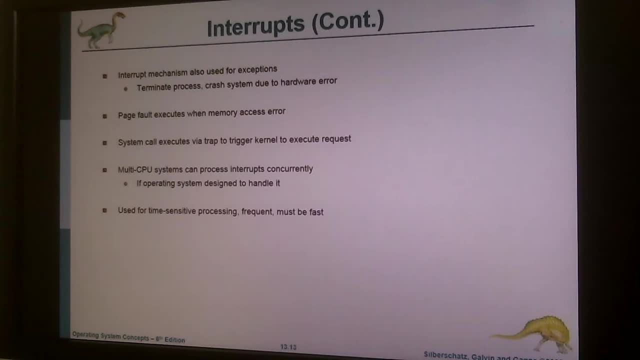 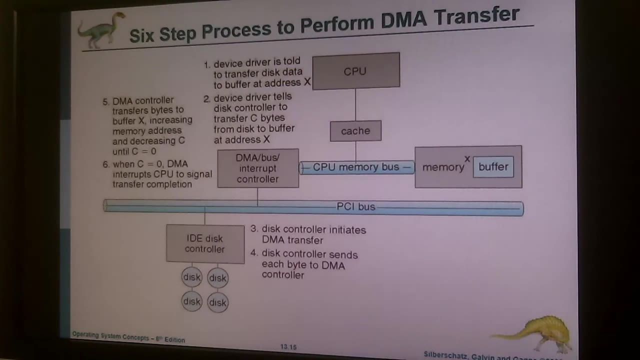 That's okay. We talked about that DMA stuff. Here's an example for that. Your CPU actually is bypassed by the DMA controller, As you see here, CPU memory bus. it says Here: as I said, DMA controller is a microcontroller all right on the motherboard, separately installed. 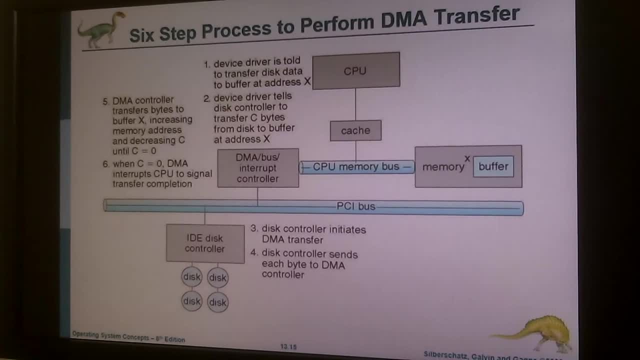 It is separate from the CPU itself. Okay, And that controller talks to the memory, the physical memory in your computer directly. all right, And your device- in this case your device is a disk- will have this device driver which access to the DMA controller. 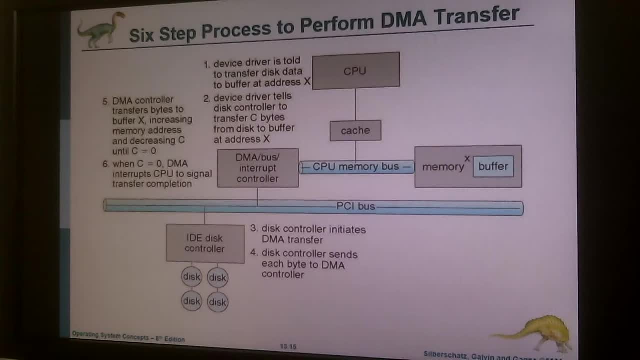 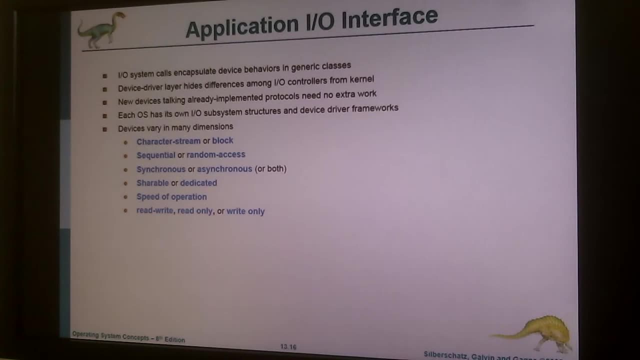 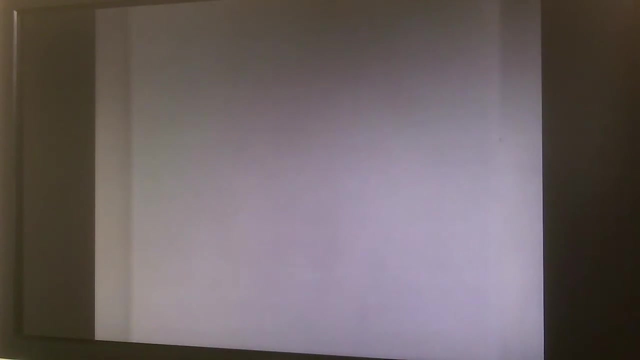 and just takes the CPU cycles, saves the CPU cycles and adds performance to your system. All right, So let me show you this very shortly. Draw it. I'll try to draw something for you. Okay, So here I have my device. 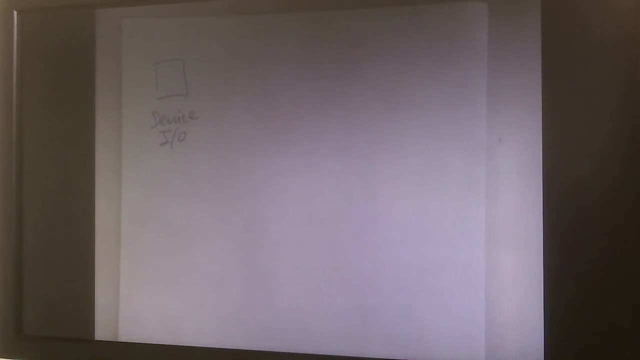 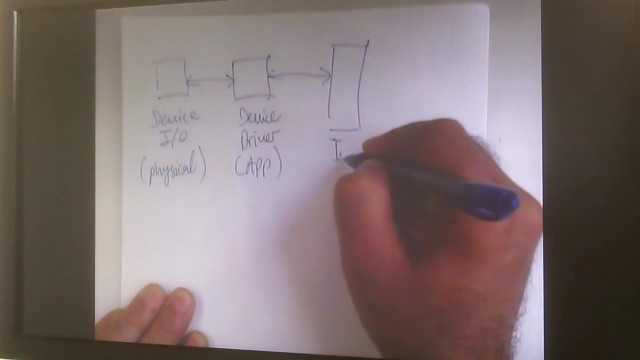 I have a device And I have the. this is physical device, right, And I had a device driver. This is an application And attached to that Now my physical device is going to be attached to the operating system, but the operating system will have an interface before that. 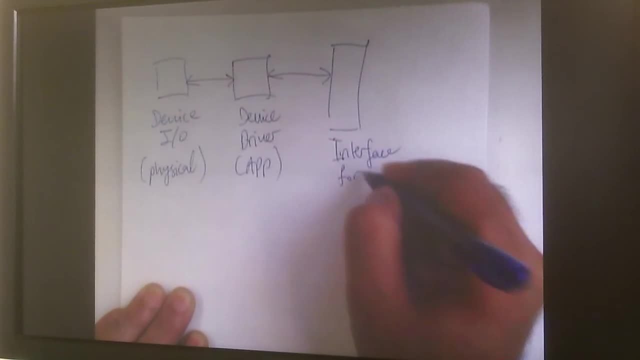 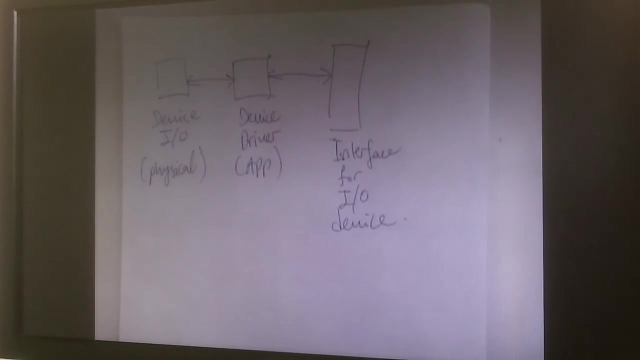 Interface for IA device. Now the reason we are having this interface. you know we have different types of IA devices. For each IA device we define our interface, like in the Java interfaces. We define methods like read, write, seek and things like. you know this kind of methods you write. 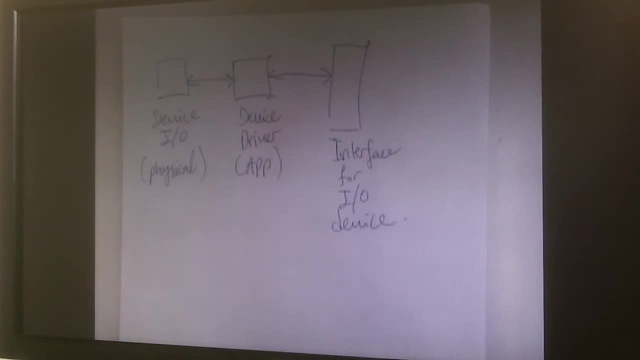 For example, you can have a method called pose in your interface And those device drivers are written to match with your interface method. Okay, It is exactly the you know, almost identical to those Java interfaces You have. you define as an operating system designer, you define your interface. 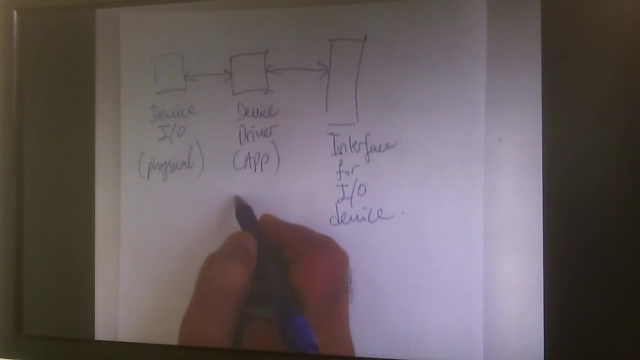 And the manufacturer fills in the methods for you, All right. They will implement your interfaces in different ways, All right. But whatever operating system you have, Whatever operating system you are working on, you should have some sort of standardization, right. 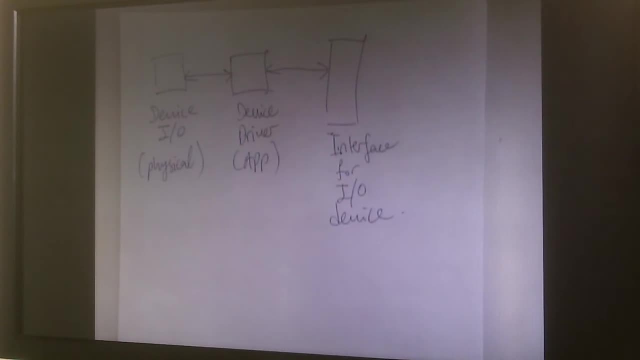 I mean some sort of standard. all the operating systems should be agree, designers should be agree So that the device- you know the manufacturers or the devices, IA devices- can implement the same interface with different methods, code in it for different operating systems. 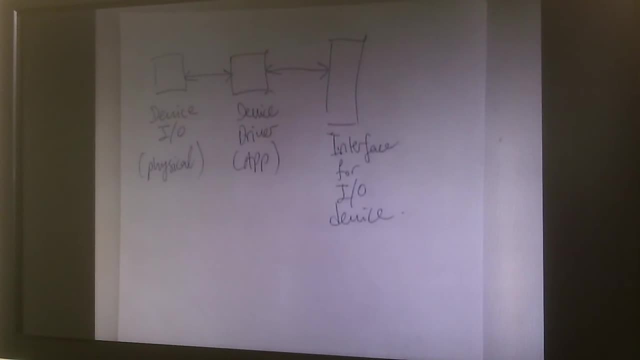 You know, if they write the device driver for Macintosh it should be almost the same. you know it should have the same interface implementation for Windows 2.. The only difference between them inside the methods. the code will change, but the methods signature will stay the same in general. 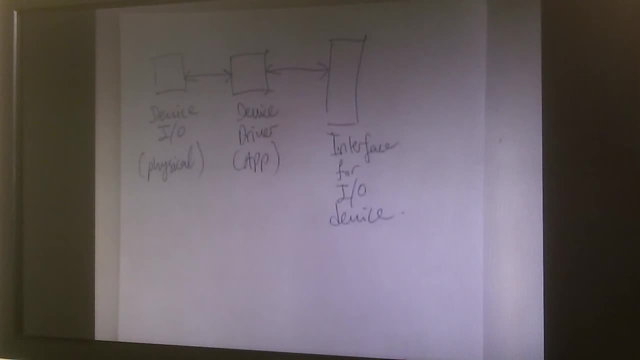 I mean, this is something we are trying to accomplish in the market. You know IEEE, ISO, things like that. They are working to standardize those kind of stuff right. For example, when you talk about TCP, IP, what do you think you know who defines the TCP? 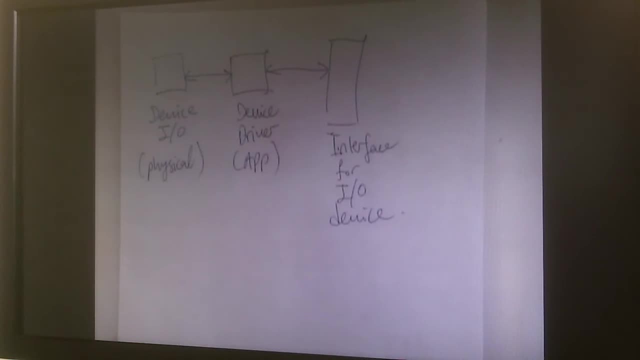 Who do you think defines the TCP IP protocol itself? It's a protocol right, But it must have a specification right. You know, for example, the bytes MTU values can be between these integer ranges Right, Or the handshake algorithm will be this and that. 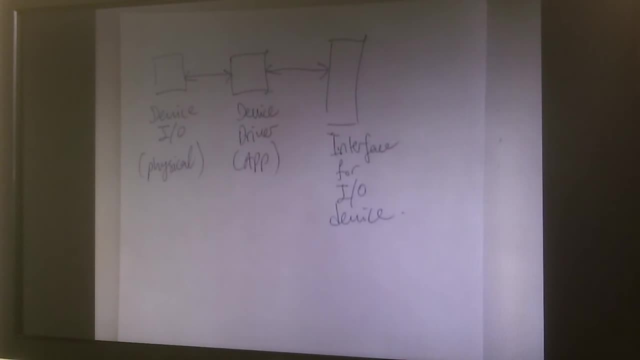 You know, those kind of stuff should be designed by someone, should be specified by someone. TCP IP is an open source networking protocol, right? And if you don't follow some specifications, if you don't have any standardization, it's going to be a problem. 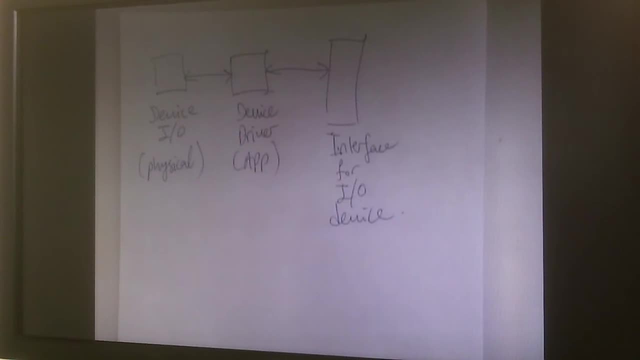 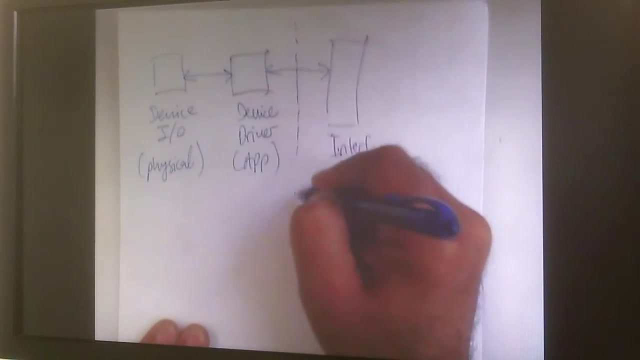 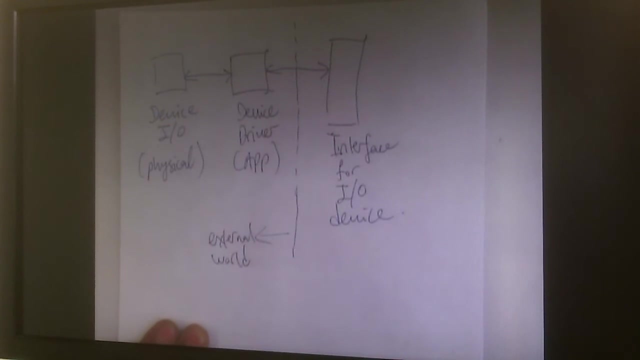 So for those device drivers too, you know you will have the interface kind of standard so that you know you can write the different drivers for them, Different drivers for different operating systems, And after the interface you know this external world. let's say: 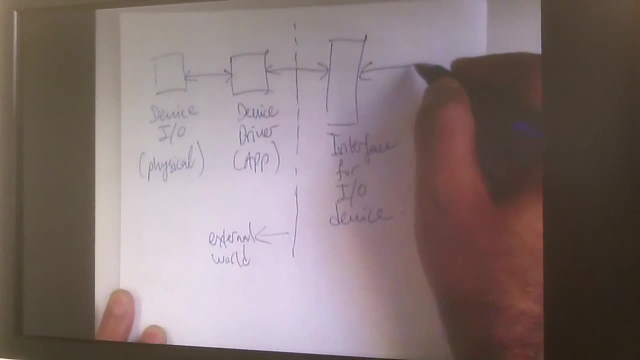 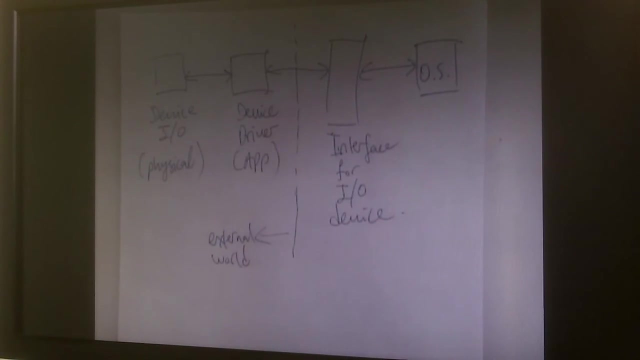 Actually, yeah, And here you have your operating system. All right, Once you define your interfaces with your operating system, you don't have to add anything else for a new device on your operating system. Right, You will not change your operating system for a new device. 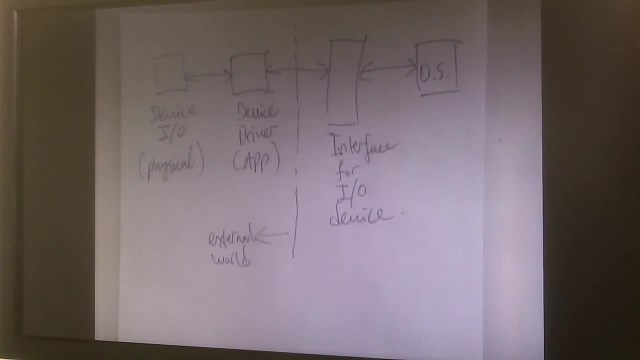 All you have to say them. you know what This device looks like, this one. I have the interface for that. So you can use this interface and write your device driver for that specific interface. So that you know, instead of recompiling my operating system, I will just take this driver, install it. it will just work, you know, seamlessly. 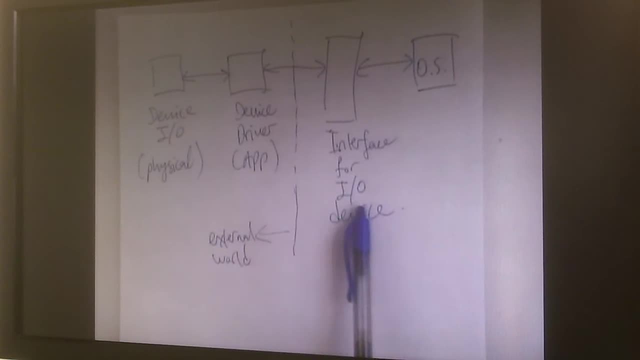 But this interface is very important for the operating system designers, You know. that is why we say: we have disks, we have tapes, we have network cards. we have what else? we have Keyboards, we have mouse, you know, mice, whatever. 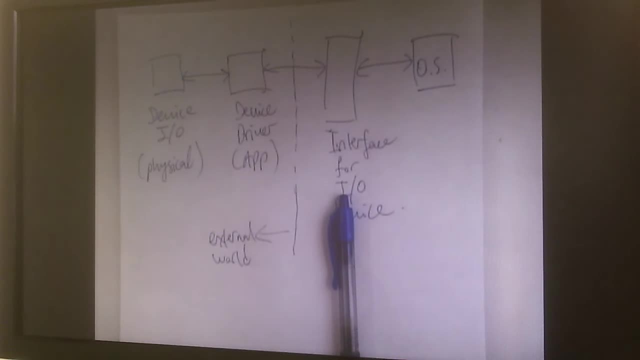 You know, we categorize and generate a full list for the interface, and every operating system designer uses the same list. At least we are trying to make them use the same list. All right, That is what we are trying to do. This is the general structure of the IO in the operating system. 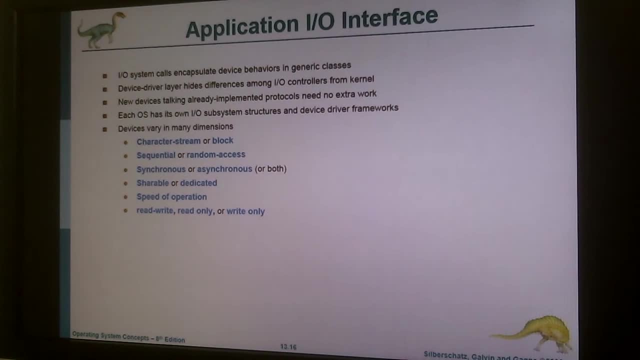 For example, this list on the screen right now. it is actually a parameter list for the interface I was talking about. For example, in that interface, some devices might have characters, Some will have blocks. For example, on your keyboard, you press a character on the keypad. 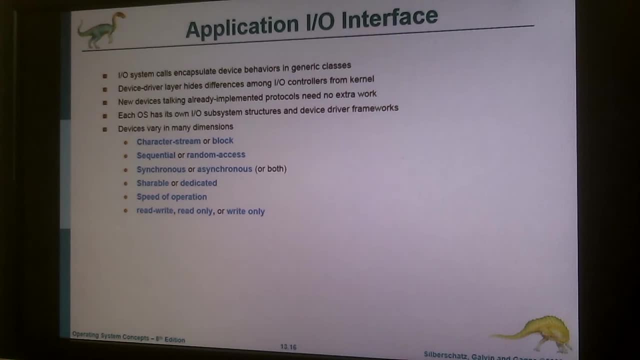 It will just send one single character, But in case of hard drive it will read stuff and send stuff to the operating system block by block. All right, It could be, you know, according to the size of the data it is transmitting. 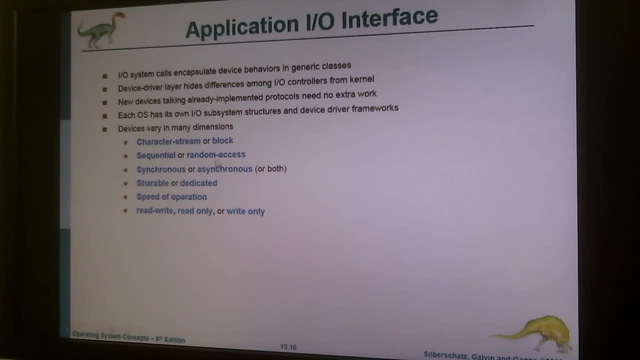 It could be character stream or block. If you are sending and receiving data from the or to that IO device. it could be a sequential or random access. The data you can get from the device, you can get it sequentially or you can get it randomly. 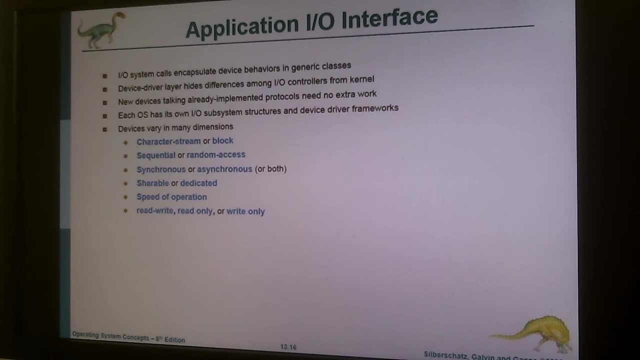 For example, you are reading a backup data from a tape backup unit, It could be most likely sequentially right, Because you can just start from the beginning and then go through right. In general, you cannot go back and forward in a tape unit. 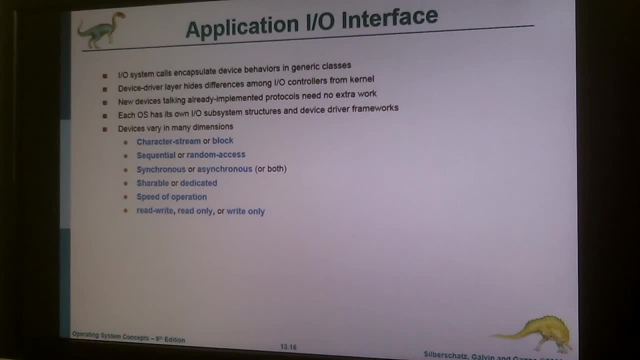 Can you do that? You should listen to it, right? You just read it from the start. Just read it from the start to the end and get the information that is sequential, Synchronous or asynchronous, or both. That means you don't really have to wait for it. 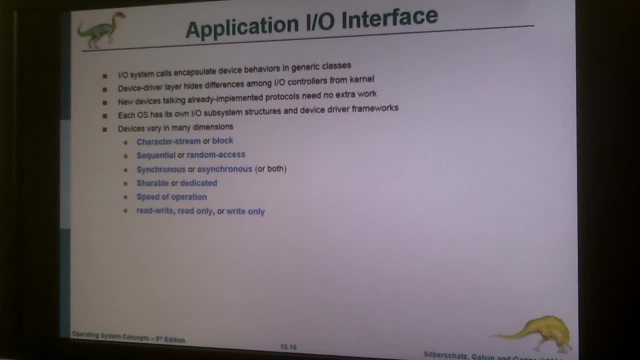 Asynchronously, you know, or more like random access style, You don't have to wait for it. But for the synchronous one you have to wait for it. You have to wait for the data coming from the IO device, Shareable or dedicated. 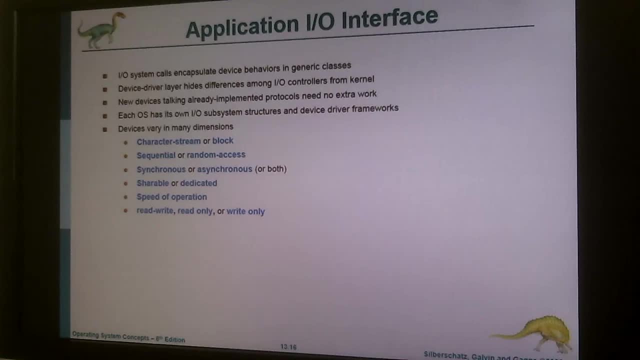 If it is shareable. I mean, these are, like you know, properties of a single IO device, a generic IO device. If it is shareable, multiple processes can share this IO device at the same time. If it is dedicated, no, they cannot. 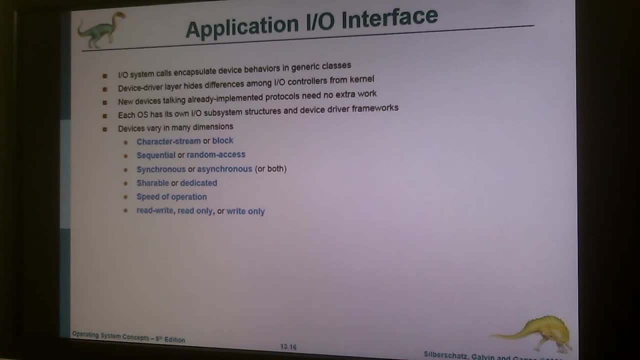 For example, your keyboard, your mouse, can be shared right For multiple windows on the screen. you see, You can move your mouse from the WinWord application to the file manager. All those processes can be activated by a left click. But some of the IO devices cannot be shared at all. 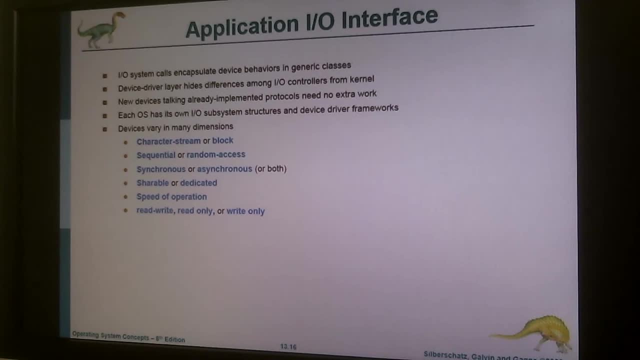 It has to be specific. For example, that network card you install in your desktop, you cannot share it. It is specifically should be used by your operating system, Not even with something else. Some other applications you have, But you know, a web client, for example, is a good example for that. 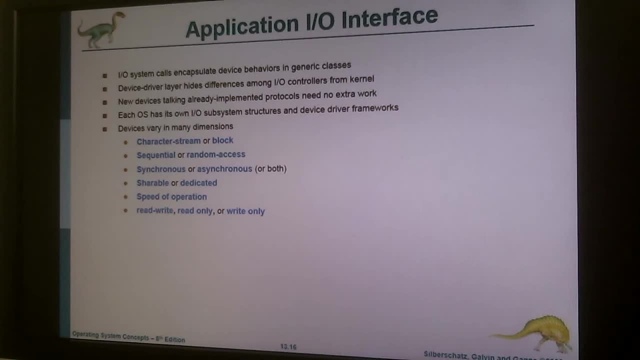 But it has to go through the operating system anyways. Speed of the operation: Some devices are categorized according to their speeds And it is going to be a parameter for the interface too. Slow ones, you know. fast ones, super fast ones, you know. 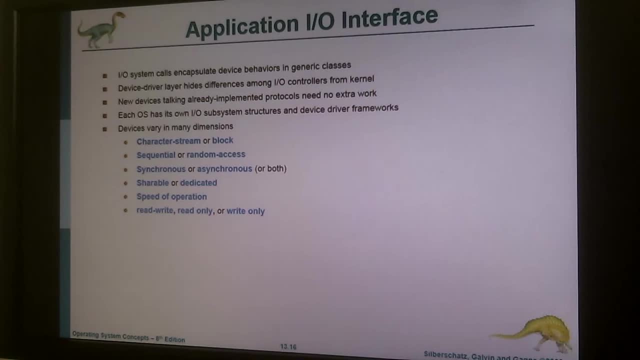 Some, for example, USB 2.0 ports. Now we have 3.0 port And we have what is that port starts with an F. It's like fire something. You know about that port on your laptop? Yeah, it is fire something. 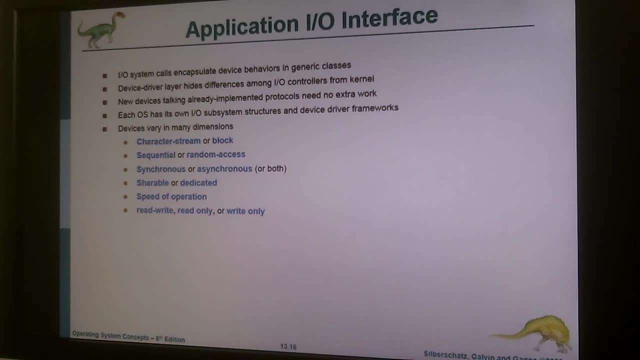 It's a new type of port. I never used it anyways, I don't know. And also, devices could be read-only. Read-only Like a random, like a CD-ROM. You cannot write on many CD-ROMs. If you buy an audio CD, right, you cannot write on them. 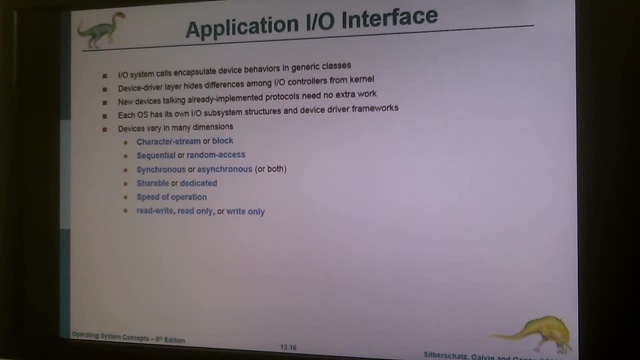 You can just read, Read-write or write-only. You know, believe it or not, some devices are write-only. You never read from them. write stuff on them. If you cannot read, what is the purpose writing on any kind of device like that? 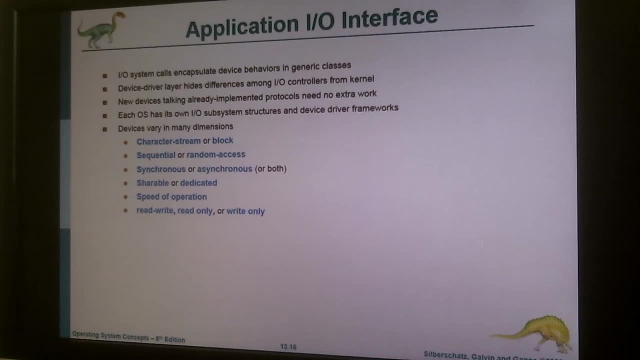 If nobody is reading, why are you writing at all? Someone else can read. What's that? Someone else can read it Or, like a different computer can read it. All right, you're going to keep that data in that device, right? 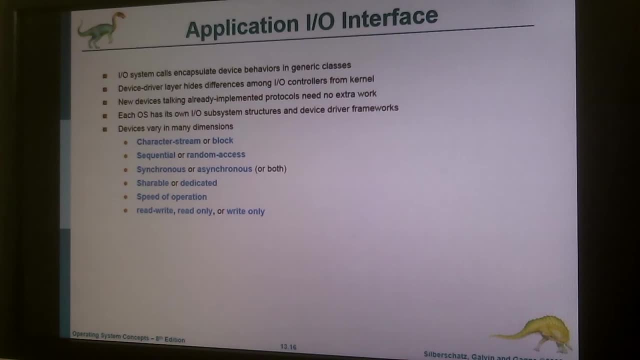 Yeah, But you never read it. Why is that? For example, think about a printer. You write to a printer, but you never read anything from a printer. right? Whatever you write, it comes out as paper, Something like that. 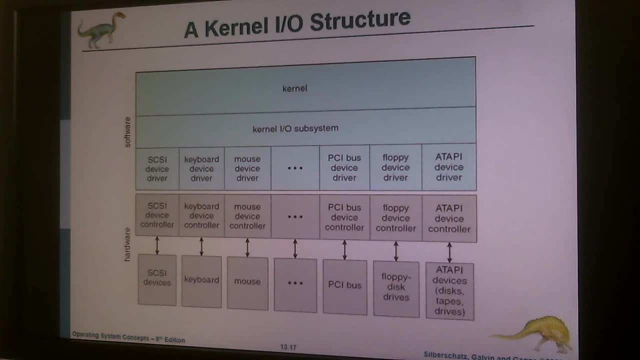 And this is the block diagram of this system that I just draw. Actually, there was no need to draw it anyways. I guess There's this kernel, the operating system itself. You have the kernel IO subsystem, which is another part of the kernel. 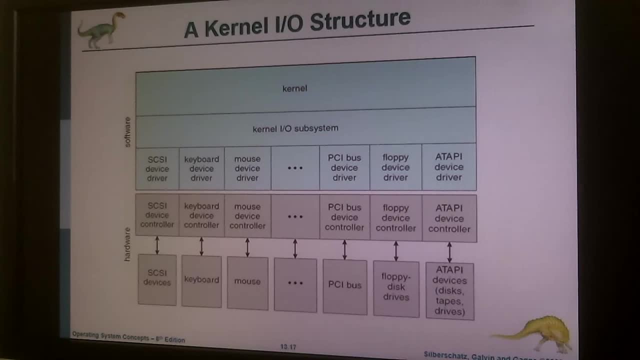 It deals with the IO only And you have drivers. These drivers are not a part of the operating system, right? They are installed after the operating system. You know, without those drivers your operating system would continue working with no problem. But, as in Windows case and Linux 2, we have some default drivers. 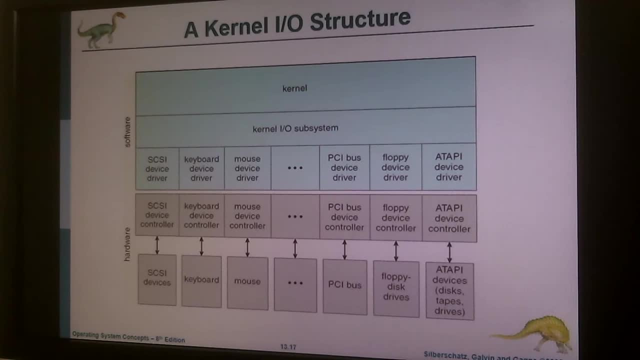 For example, most of the you know the mouse, wired or wireless. they will not need any driver at all, You just plug it. it will just work with no problem at all, Because you know these are very common devices. 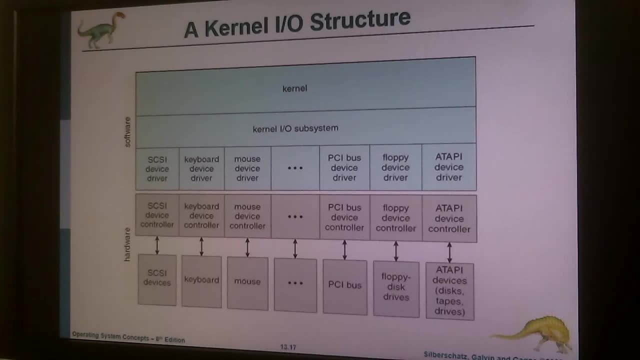 Many people have them. you know Thousands, millions of people are using those kind of stuff. So operating system designers say: you know what, Since everybody is using you know, like 80% or almost 99.9% of the laptop users are using mouse. 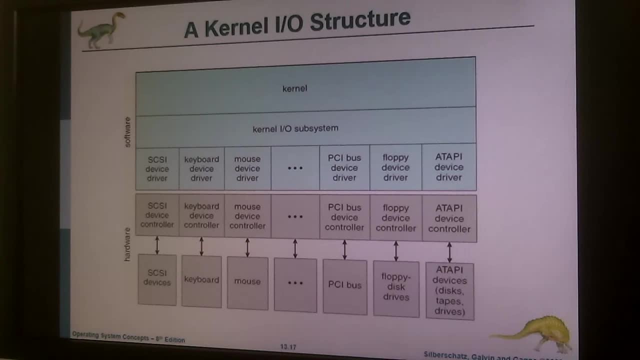 let's put a mouse driver in it, So you know people will not cry aloud trying to download, and you know, install a mouse driver for that. Anyways, we have the drivers And we have the controllers. As you know, every physical device is a bunch of mechanics, electronics. 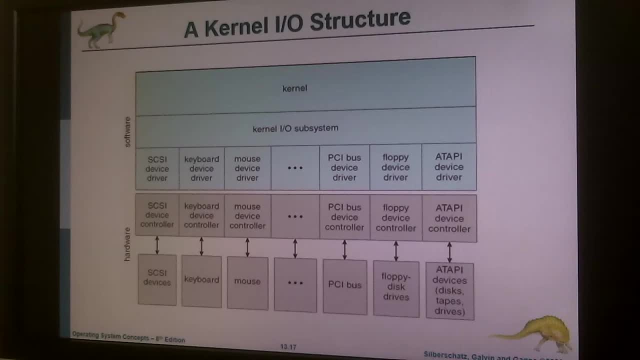 So they really need a way of communication electronically. So they have the controller boards, PCBs. These are controller boards or microcontrollers with a firmware on it. And finally we have the physical devices right here: A SCSI device, a keyboard, a mouse, PCI pass, etc. 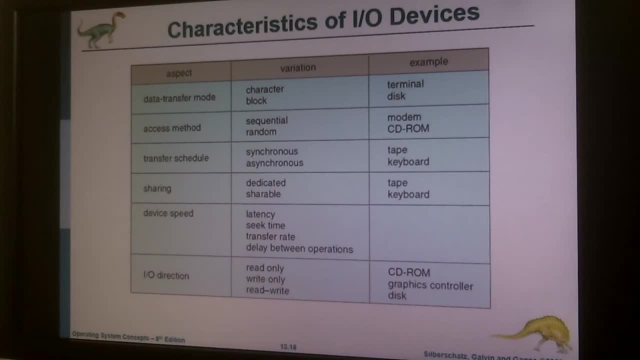 This is the general structure characteristics. Well, again, when you're designing your interface inside the operating system for the IO devices, this could be another set of parameters that you should use, For example, what kind of transfer mode you're going to use. 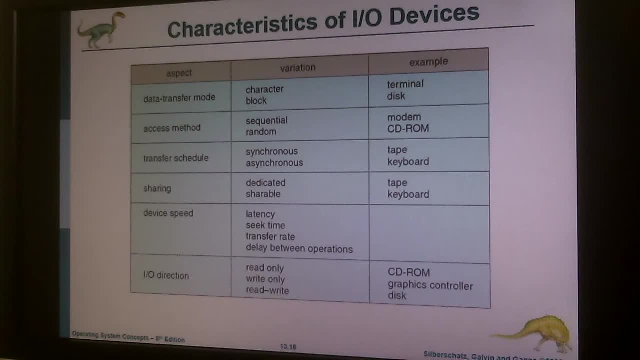 Is it going to be a block or a character? And an example for that terminal screen. Terminal screen, you know, even in Macintosh you have one. Right In Windows you have this black and white command prompt. You can actually change its color. 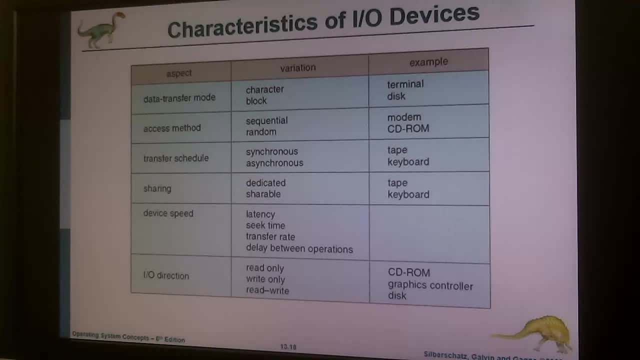 I always make it green and black. You know it's like the matrix style. huh, I feel better. No, the truth is, in 1980s we had those dump terminals, workstations, And they had like two or three options. 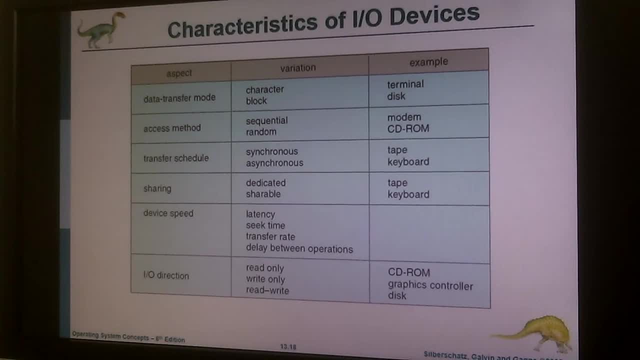 The first option was green and black, The second one orange and black, believe it or not- And the other one was white and black, Black and white. in other words, We had all those green and black ones and I liked them very much. 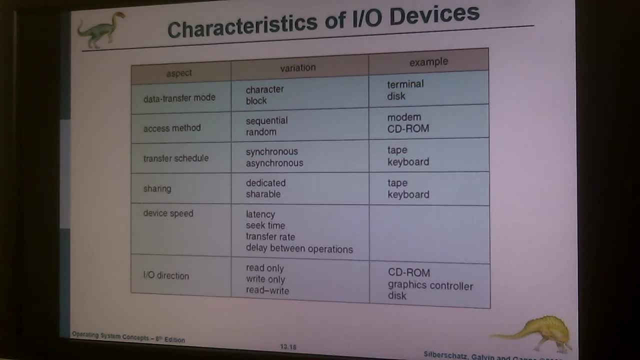 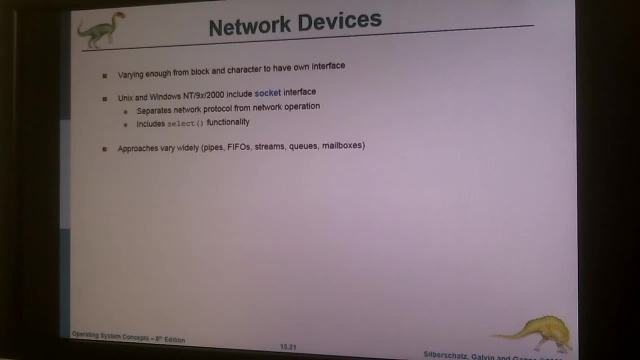 Anyways, device speed, IO direction, etc. Let me see if there's any other important stuff here. Okay, network devices. Okay, when you're talking about hard drive, what kind of information your operating system or your application sends to your hard drive? 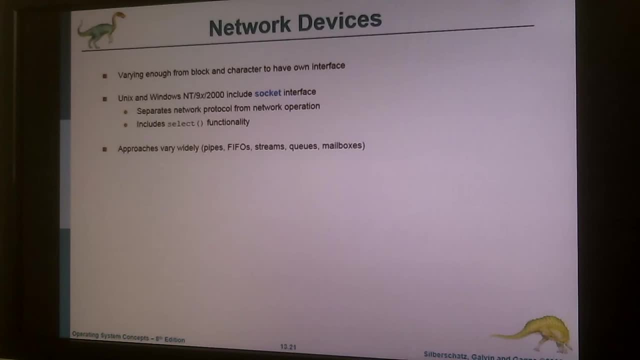 Does it say? you know, I actually asked this question before, when we were talking about processes. Do you think you tell: okay, you're trying to open the testtxt file, right? Do you tell your hard drive to give you the testtxt file? 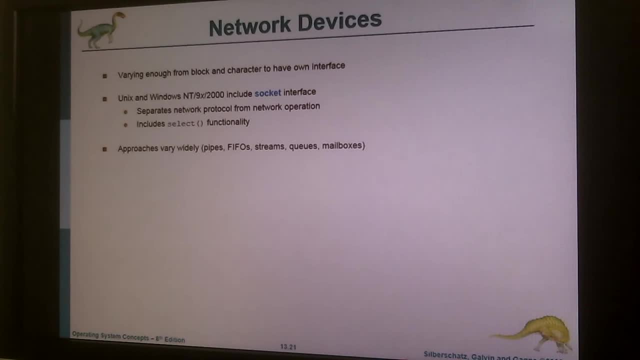 or you tell it: give me that block on that sector and track. You have two options, multiple choice. A: you just give the file name. B: you specifically give the location, the sector number and track number and things like that. 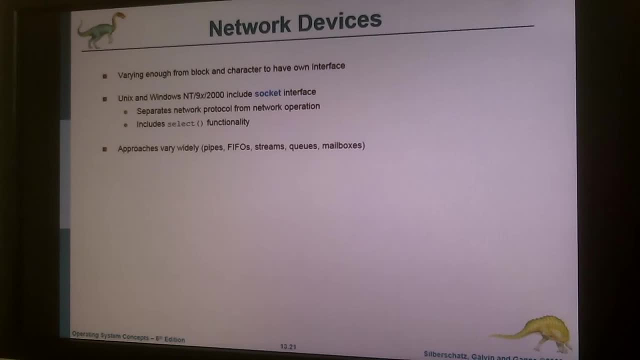 A block number, in short A or B. Who tells A? One student here: Anybody: always bring A. You say A, No B in this case. The rest, Oh. some people say none of them. Wow, it's interesting. 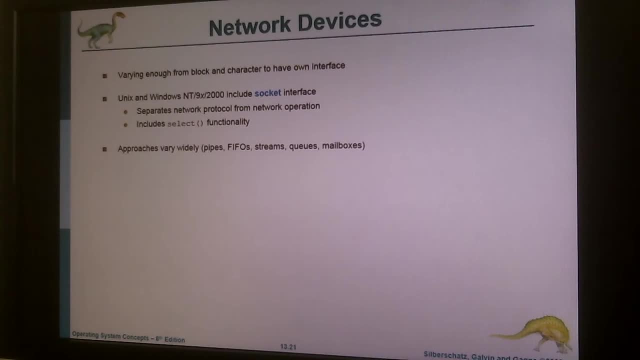 Well, in general, your operating system doesn't have any idea what is in your hard drive, which files are in your hard drive, all right, But it will have the idea when you first reach your hard drive and get the list of. That means that the file list should be somewhere in your hard drive. 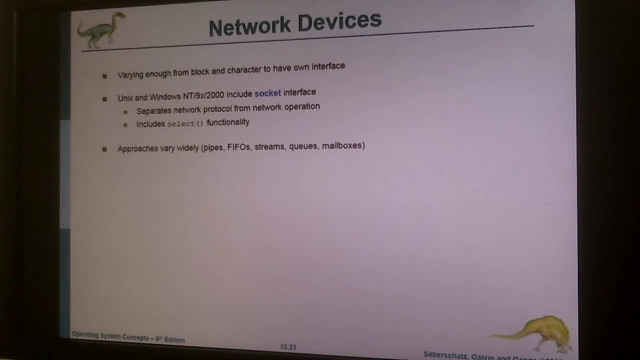 the file structure, subfolders, folders. Remember that root structure, one level, two level, directories, That tree, the folder structure Has to be somewhere in your hard drive. In that case you unplug your hard drive and go and plug it to some other computer. 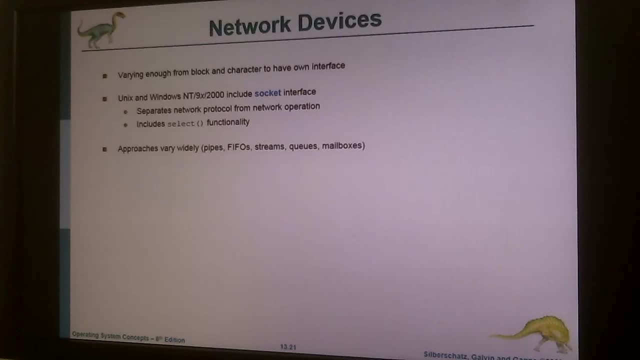 you will see the same structure, right, Nothing is gone. You have that same structure, same table, same director structure, because you got that table in your hard drive. That means your operating system just says: give me text, test, testtxt file. 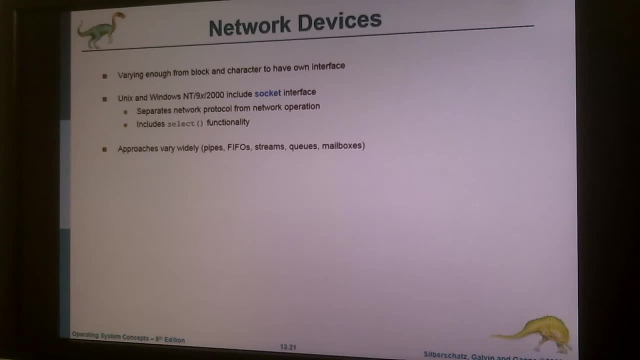 It just tells the file name. It doesn't have to say how, to know anything about the blocks or anything. It will just say: give me the file And then, since the hard drive itself has this controller board, the PCB board, it has the ability to convert that file name to the blocks. 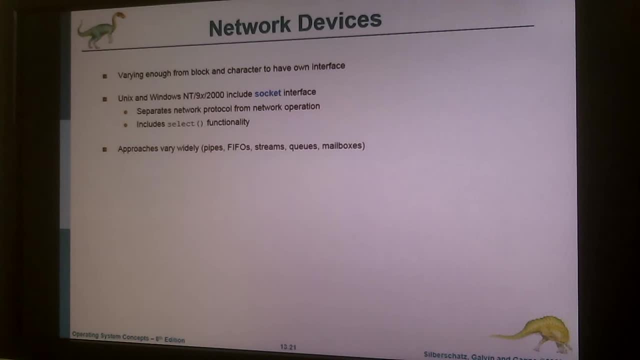 And it will just read the blocks and then push it into the operating system And then you will get that data For the network card. you can read, write from the hard drive, right, But what are you going to do with the network card? 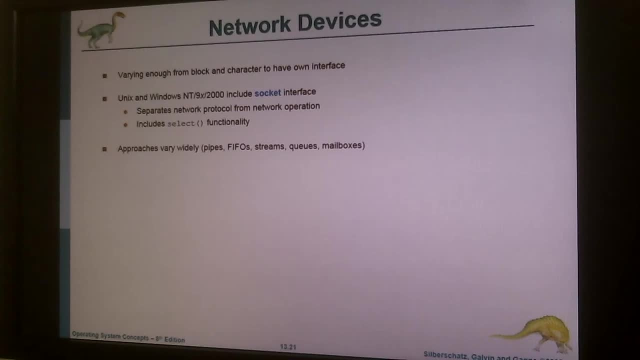 Both of them are IOD devices. Can you read from a network card? Can you write to a network card? Can you seek? Do you have a directory structure in a network card? Well, many of the operations are not identical, but some of them are. 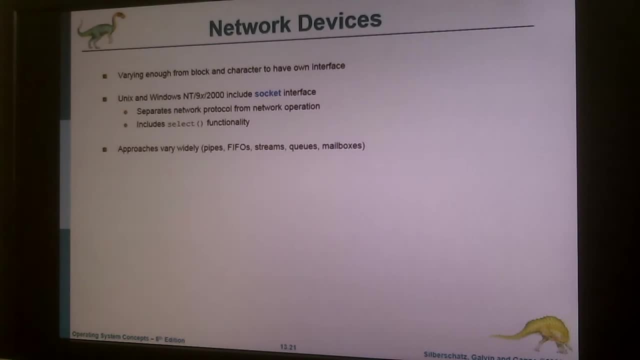 You can actually read from a network card, right, How It is called listening. You know you can listen to a network port for a specific information. For example, you use your web client, your browser, to connect to NYITedu. 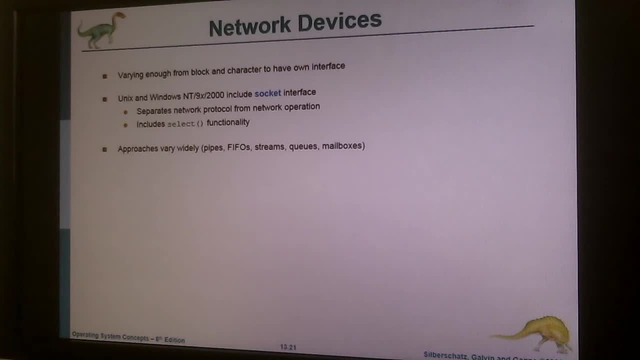 That data comes from the NYIT servers. You're actually listening your network card at port 80, right? You just listen to port 80. Whatever comes, you show it on the screen on your web client, On your browser. That is called a socket, actually. 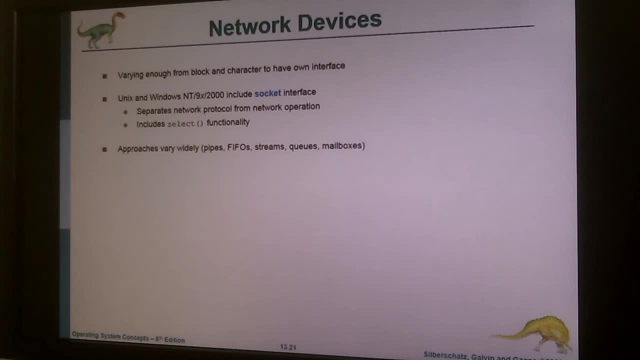 You can reach to your network card through the sockets and it uses the port numbers. All right, There's another IO service, let's say Clocks on time timers. The operating system has this ability. It uses crystals and digital integrated circuits to generate clocks, clock ticks. 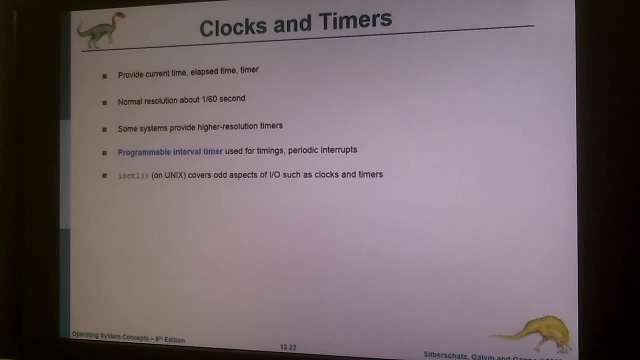 And those clock ticks are used as a timer. You know, you set your timer to 10 milliseconds and at the end you spread a lot of interrupts everywhere, for example: All right, You can do that, Or just give me the system clock. 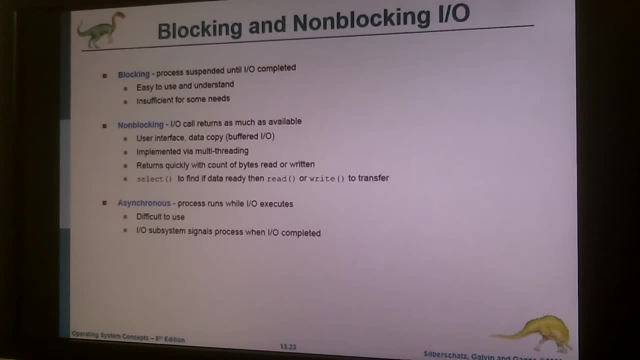 Okay, Let's see Programmable interval timer. Yes, sir, Okay, This difference differentiating between the blocking and non-blocking IO devices are important because some of the IO devices you know when you're programming you can. 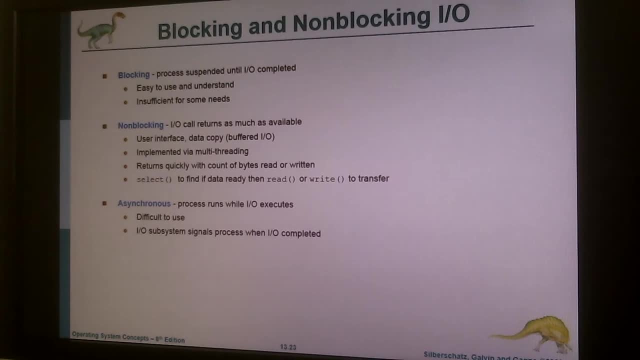 use threads right. Those threads will give you parallel programming ability. you know, at the same time you can do multiple things and if you have more than one course, you can take advantage of them. you know you can boost up your applications performance, but some of the devices will not work with your. 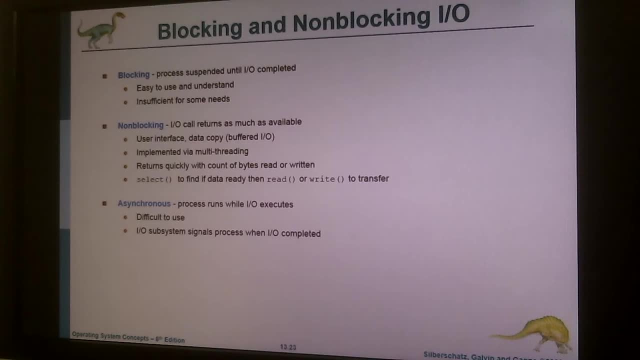 threading approach because, whatever you do, you cannot access multiple times on that IO device. or, when you ask for data from that specific IO device, you have to wait for the answer- alright, some of them are blocking your process. so you have to wait for the data, okay, but some of them are not actually blocking you. 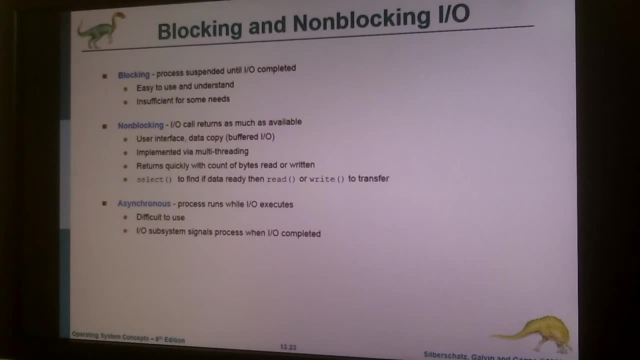 know you don't have to wait for it, because it uses something special called buffers inside it and also a part of your main memory, your physical memory, can be used as a buffer. by the way, you need to know about buffers and caches. you know there are different things and you should know the difference between them. I'll talk about. 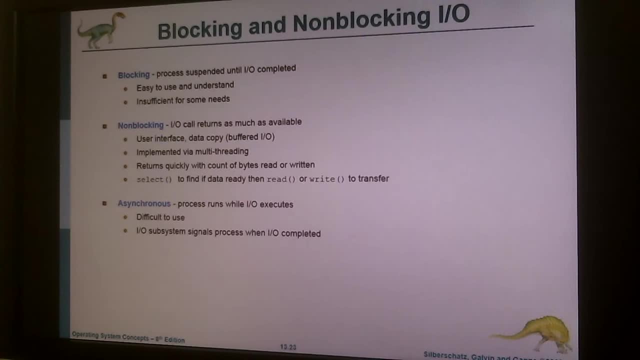 it soon. okay, on a non-blocking I-O device, you just tell: give me this and then continue. whatever you're doing, it will just read it. you know it will not stop your process as the blocking one does. it will just continue working on the data. I will. 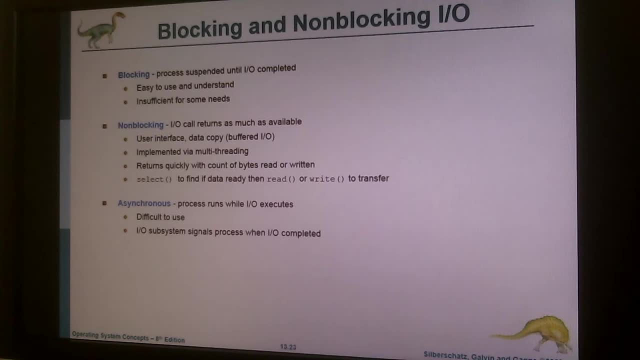 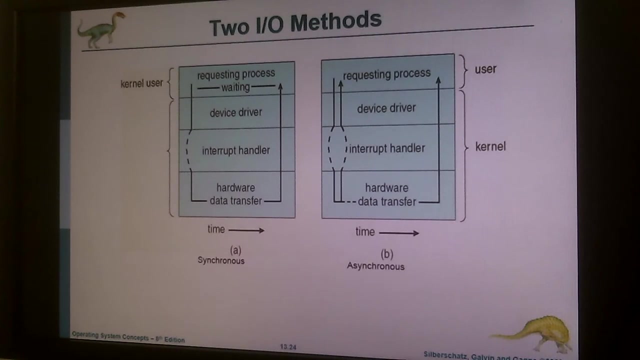 put it in a buffer and then your process will read the buffer at the end and it will just continue working, continue executing. all right, asynchronous I-O devices are not really used because it's very hard to code. you know, if the implementation is hard for the developer, it's most likely not going to be used. all right, oh, we need to talk. 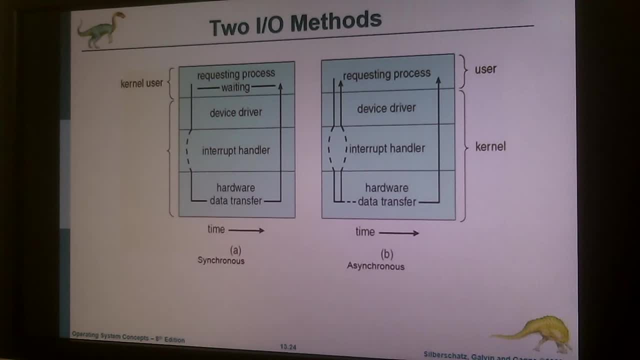 about the caches. buffers are like queues. you remember data structure queues, right? queue is something that you put multiple things, data, process whatever objects in order and then start processing them from the beginning. all right, from the first one. that is a queue. so buffer is a copy of an original data. for example, you're sending hundred pages. 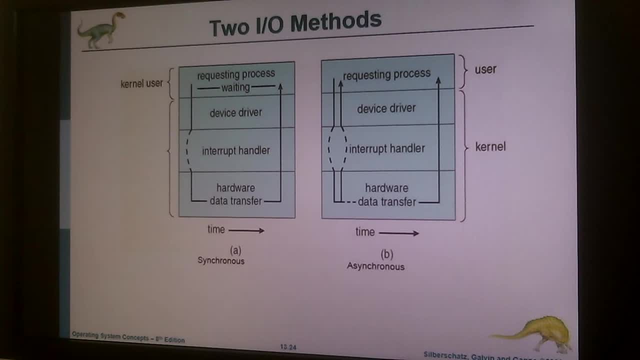 on to your printer and your printer's memory is two megabytes and each page you're sending is two megabytes. What happens? You receive the first one and you have to wait until it prints the other one. right, And then, once done, yeah, your. 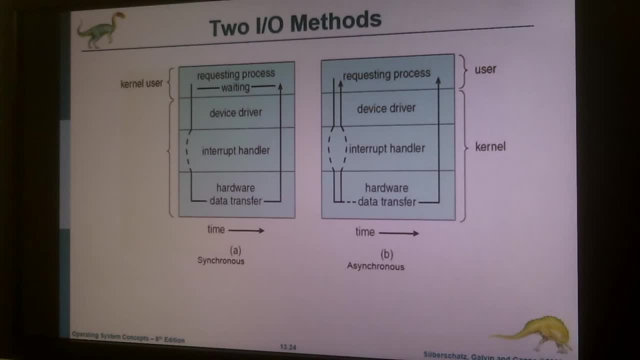 operating system will send the other one and while it's waiting, where it really waits- I mean those 20 megabytes, right, 18 megabytes of it- will have to wait somewhere, somewhere in the operating system, right somewhere in the in the system, in the computer, in the hard drive, in the memory. where does it wait? that's? 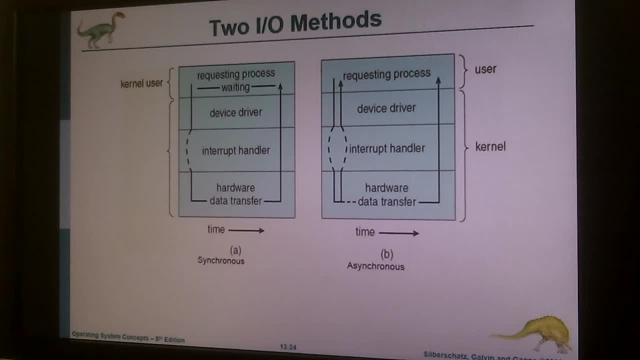 kind of it. it has to wait in the actual memory because you know it is being processed. since it's being processed, you should always keep- I mean, the application will always keep that alive- data on the memory, since in turn it will be processed. but some printers have internal buffers, it doesn't matter. 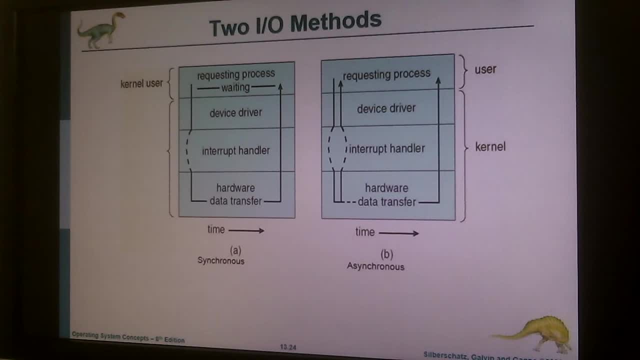 how many files you're sending it just keep it keeps taking them. you know it doesn't. you know it has a large. some of them actually have hard drives. some printers- you know some copy me, xerox copy machines. they have hard drives, believe it or not. they have an operating system too, of course. you. you're pressing. 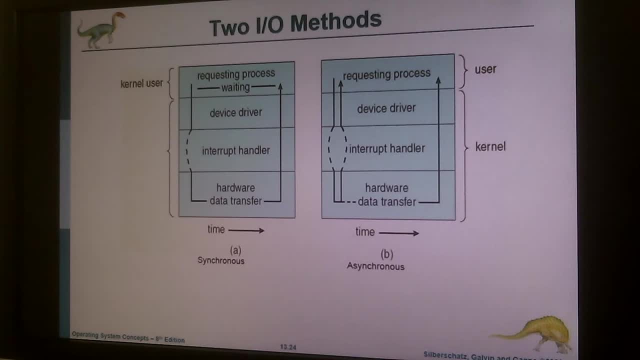 those buttons. it's coming from somewhere, right? I mean seriously, yeah, it has an embedded operating computer and an operating system, right, and what the files you're sending goes into the internal buffer. that means you're copying some stuff into some place, into some queue. that is buffering. caching, however, is not copying, it's the original. 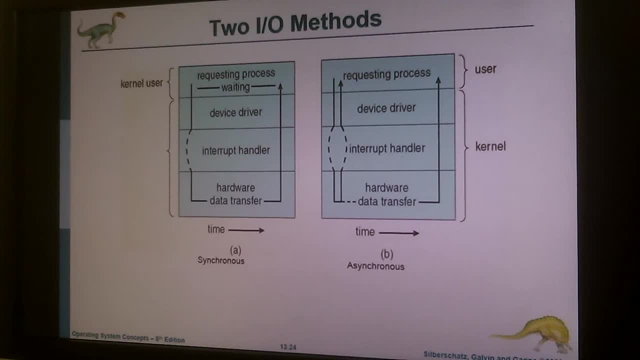 data itself. you're just moving that data, not copying. you're moving that data into a cache, which is a super fast memory. right, it could be on the physical memory, but most likely it's gonna be one of the caches in the CPU: l1, l2 caches. all right, there's something wrong with. 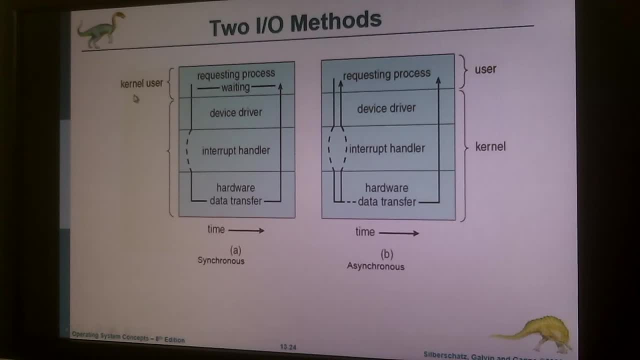 this picture on this part here, that kernel word supposed to be right here, and this is two IO methods, synchronous and asynchronous. synchronous has to wait. all right, there's a request for the from the IO device: read or write or seek or listen, whatever. I mean some sort of request from the IO device and of 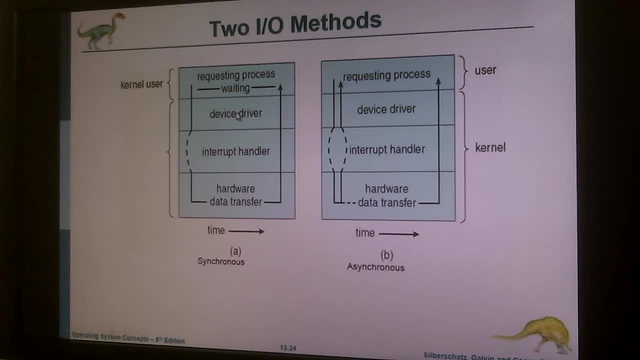 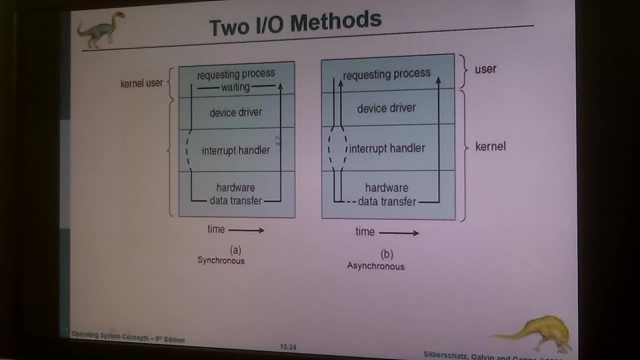 course it's going to be taken care of by the device driver, and that device driver actually generates the interrupts and then data transfer completes. but while these are being done, this is the time your process has to wait. all right, it starts here, works his way out here when it's ending. in the meantime you can't do anything. you. 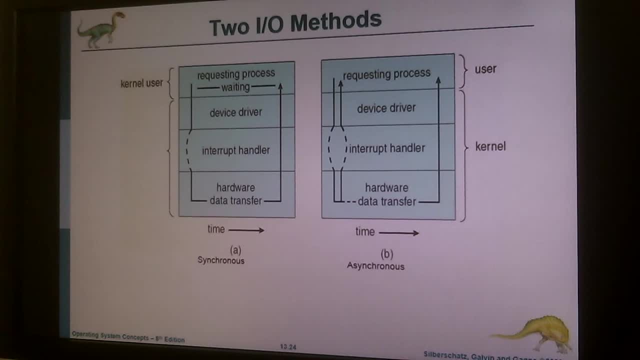 have to wait for it. all right, well, actually, that you can do something, because you can just put the process in waiting queue and then you can switch to another process by using the CPU scheduling. but if your IO device is asynchronous, in that case you don't have to wait for it, you just say you. 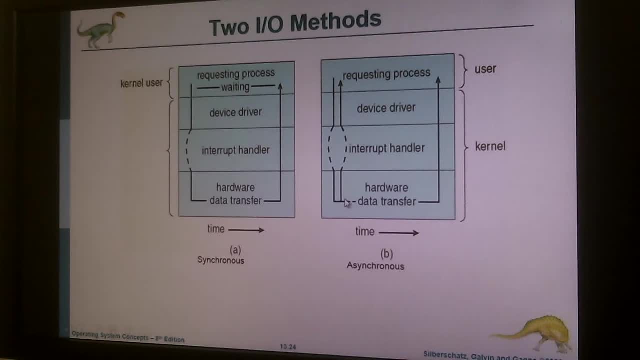 know, give me that and then it will take care of it. it will just put it in about buffer and you can actually continue running the same exact process: execute, continue executing. but that's a process must be able to go back and read the data from somewhere you know. if you say, for example, you can write a 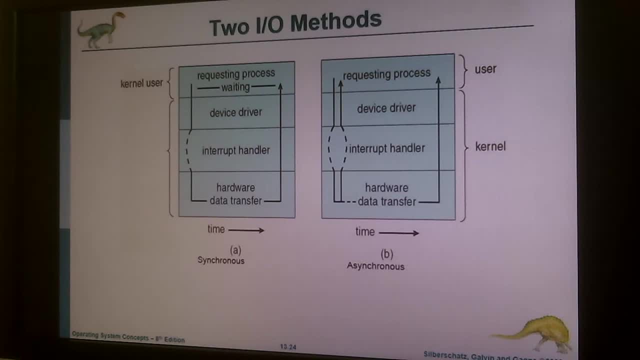 read from hard drive method in two ways. first way: you can say: you know, give me this file, open that file. I will wait for it. the second way: give me that file, but I'm not going to wait for it, I'll do something else. but 10 milliseconds later. 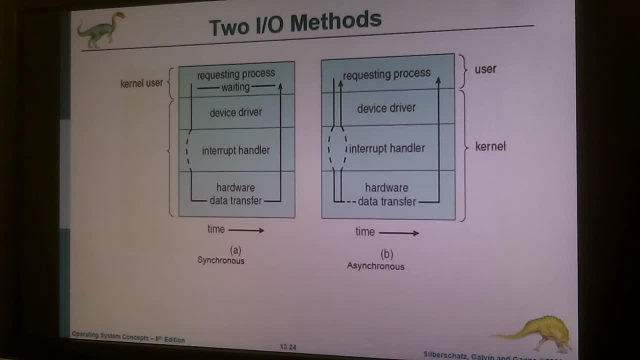 I will come back and check if you had a file already or not. I will check the buffer. all right, that's another way. so this is the second one is asynchronous. you don't wait for it, you do something else in the meantime, your process is doing something else. 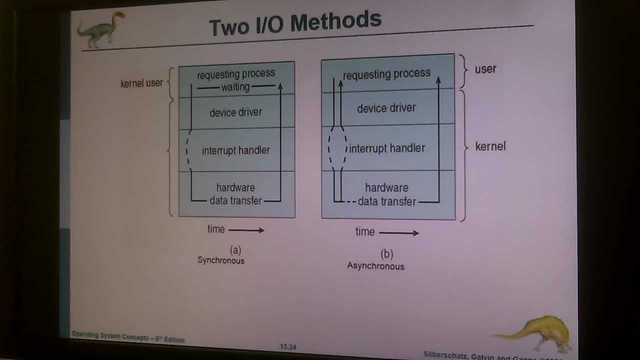 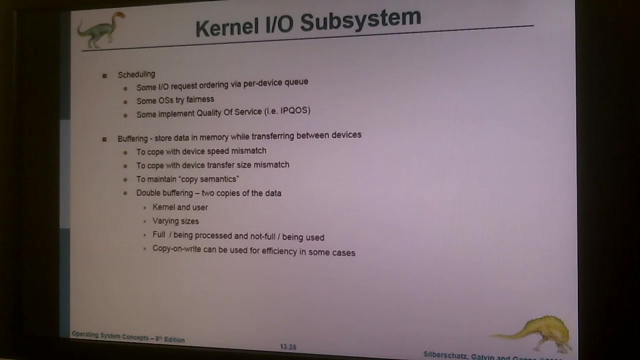 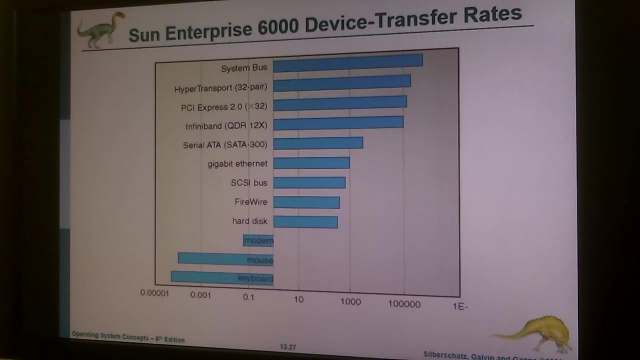 you're not actually giving away your process and you know it will be put in the waiting queue or whatever, but you yourself, the the process itself, does something else in the meantime. okay, so that is called asynchronous. this is a comparison for the server rates or different devices, some examples actually, if you look at this. 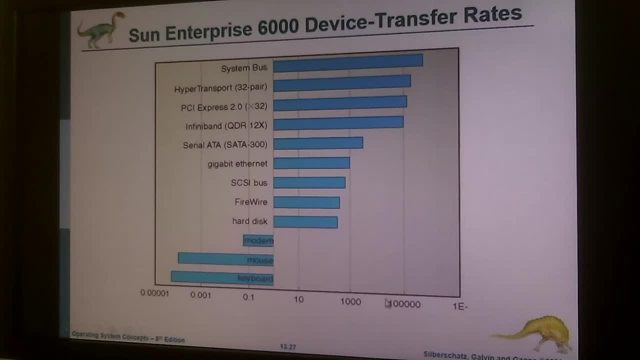 one it starts, the here is zero, and which one is the fastest? one is the system bus, and actually CPU itself is way faster than the system bus. but in this diagram data then somehow for some reason they didn't include the memory and the CPU in this list, because 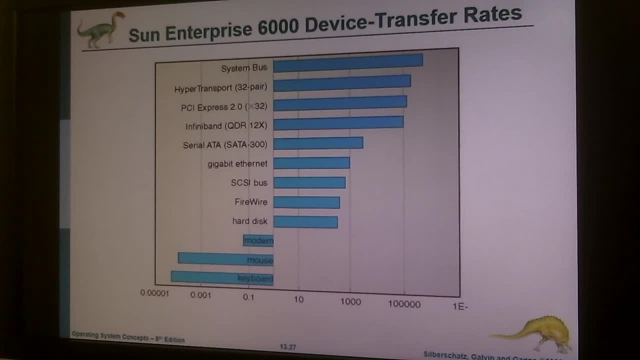 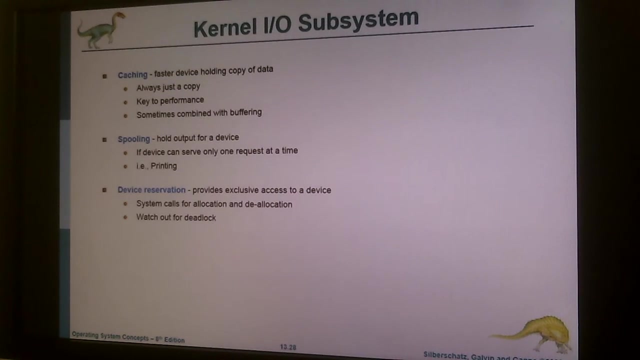 I think they are trying to tell us: hey, system bus is the IO bus and the rest of the stuff I'm putting here is IO related. you know, CPU itself isn't, is not an IO device. all right, caching, spooling? well, spooling is exactly the same thing. we 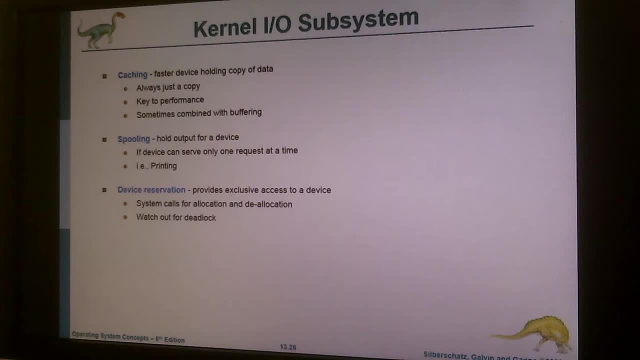 spooled a service for your printer. I'll show you something. I don't know if you haven't seen this before or about how can I do that. press this, ok, go to your Windows Computer. if you have one laptop here right now, I don't know if I can see. 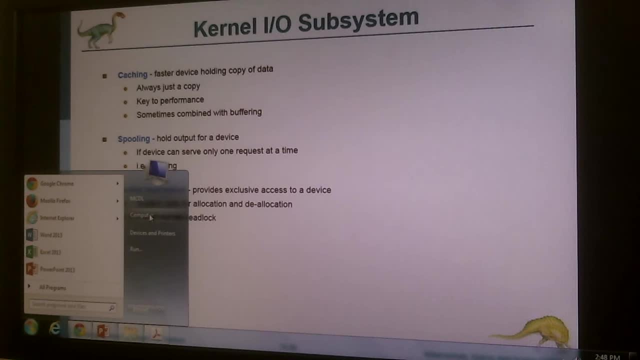 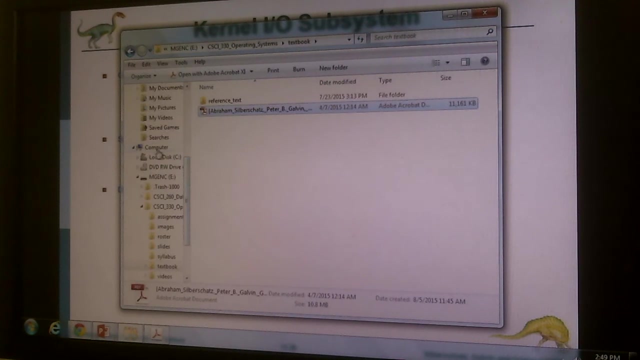 it here because of the restrictions of the system, but I'll try it anyway. as you see, my right click is not working. I hate you. okay, try another way, and if that one is not working, maybe this one is gonna work, and probably not. oh really, this is crazy, see. 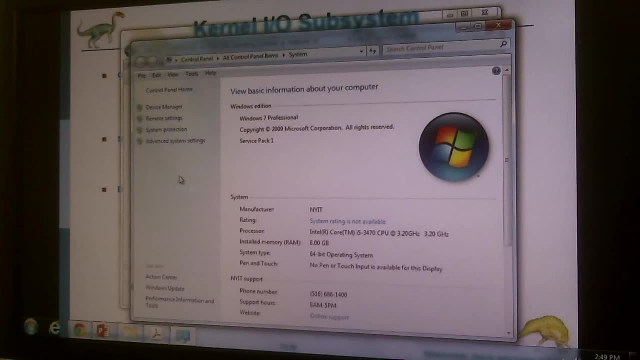 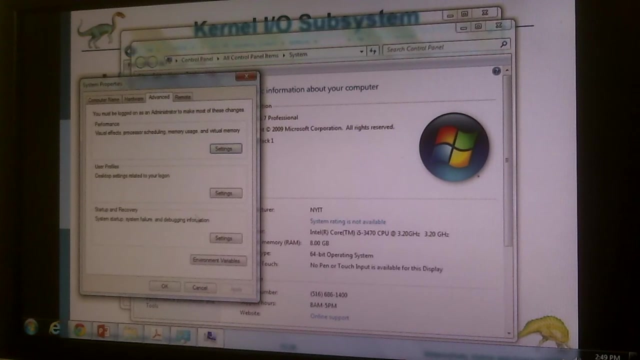 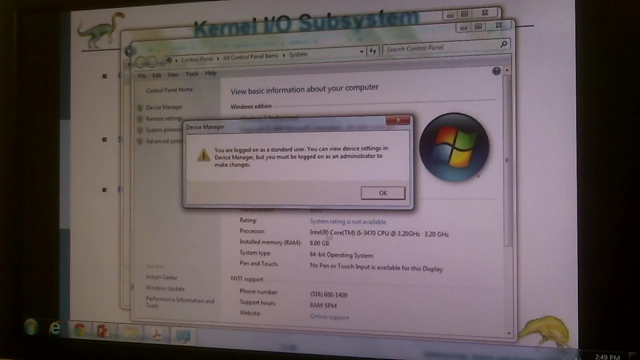 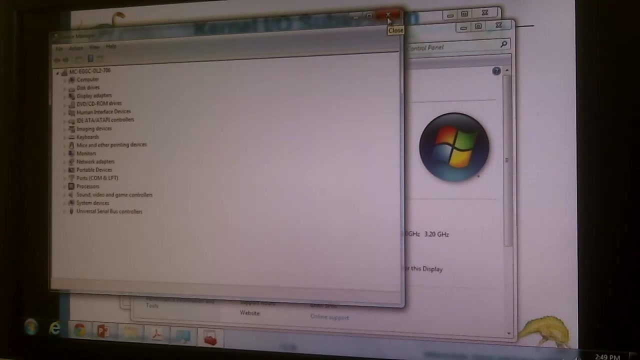 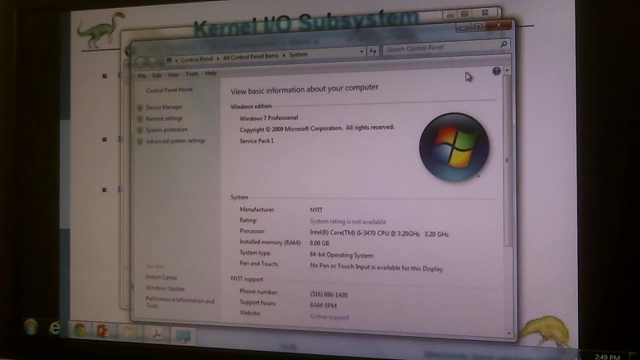 that this is not a good thing. what I was trying to show you right here. I do have system settings twice manager. no, no, well, you don't have your rights. okay, you cannot change, but you can see it. you know, you can watch it, but it can't touch it. okay, I was trying. 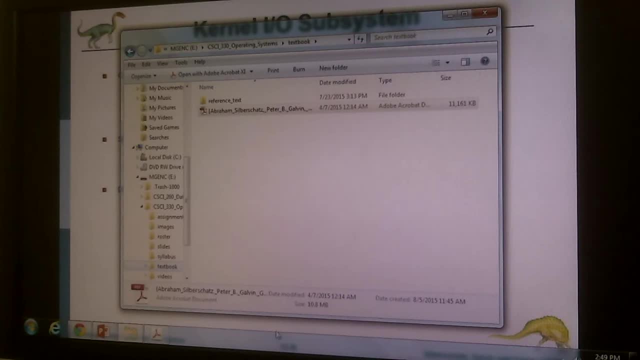 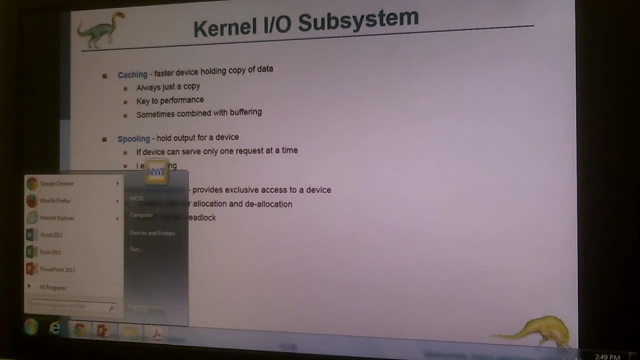 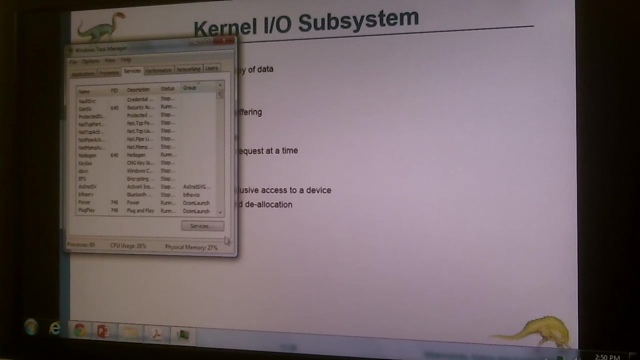 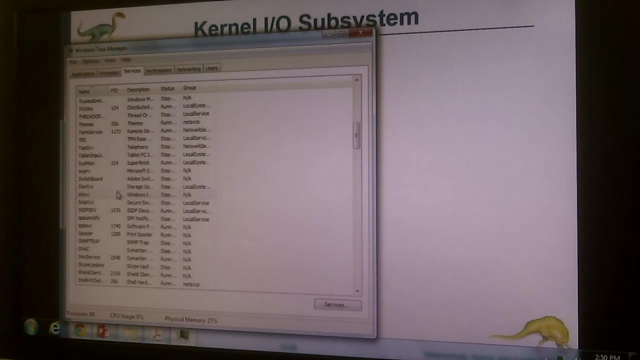 to show you how to change the system settings twice. manager. no, I don't know how to do it. show you, alright, let's one more try, maybe i'll see it here. there you go, you see that print spooler. and there's actually another way to go through my computer and properties and 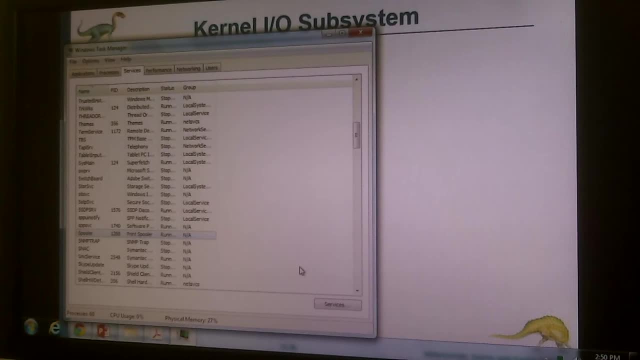 services, etc. but this is a service running called spooler in windows. it's been the same for like last twenty years. they use the same way. uh, if you stop this print spooler service, you can actually, you know, uh, kill the service or stop the service. 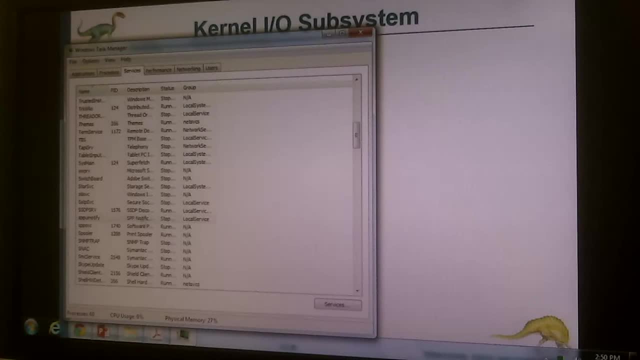 starts, etc. you know, uh, if you stop it, you cannot print on the printer anymore, even though you have the driver, you have the software, you have everything. but if your operating system, spooler, is not working, that means the queue is not working, queue manager. so you cannot really do anything. 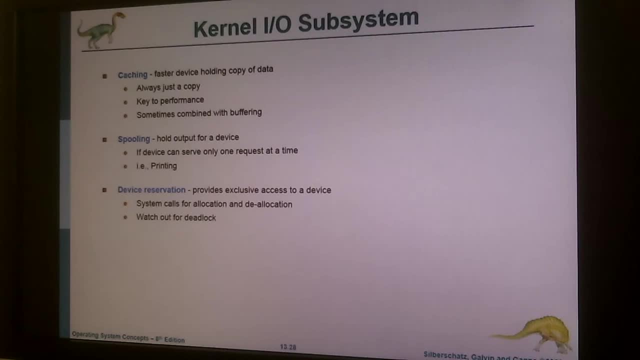 anyways, spooler. spooling actually is a system, is an algorithm that we use to send data to our devices like printers. alright, caching is also another one. uh well, caching is copying, buffering is moving. don't be confused. i think i said the opposite. i'm not sure. 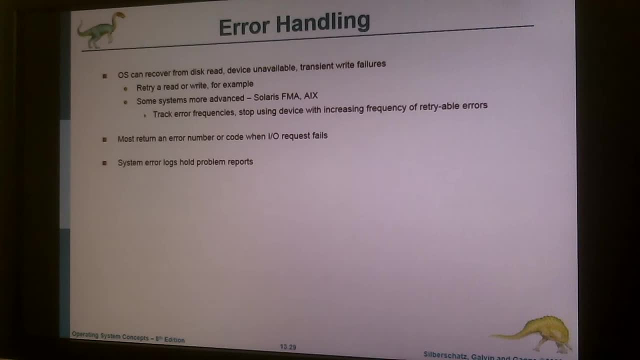 by the way, when i was talking about the interrupts, i was saying that you know you have two types: masking and non masking. also, there are other ways to manage interrupts by changing their priorities alright, for example, for offer system calls and system related operating system related, journal mode related. 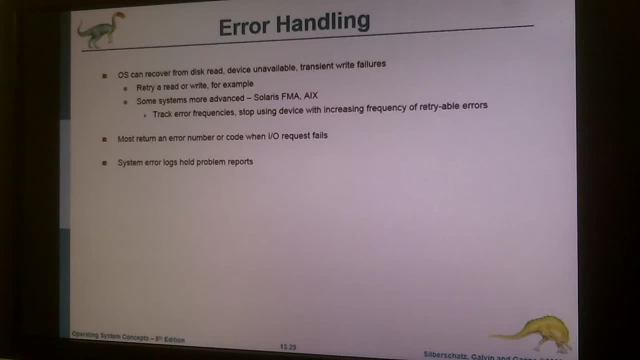 processes. you can change the uh well, uh uh. the priority level is higher than the user mode processes because you know you have to take care of the house at first and then you take care of the storage of the pirn, the, you know, the neighbors or whatever. so most important part is the operating 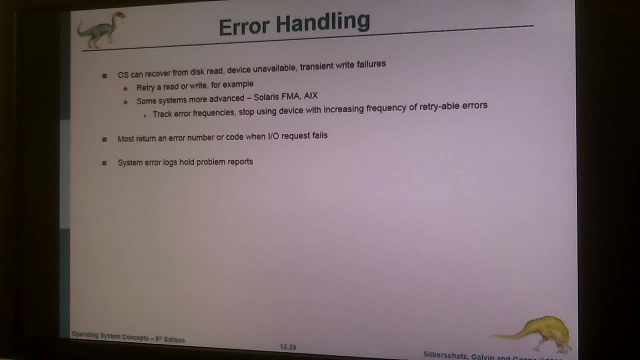 system first and then the user applications. so I need to say that: error handling. well, those interrupts are used for error handling too. if there's an error with your iAdvice, if you cannot read, if there's a bad block, for example, in your hard drive, what are you going to do? if you cannot read it, you have to. 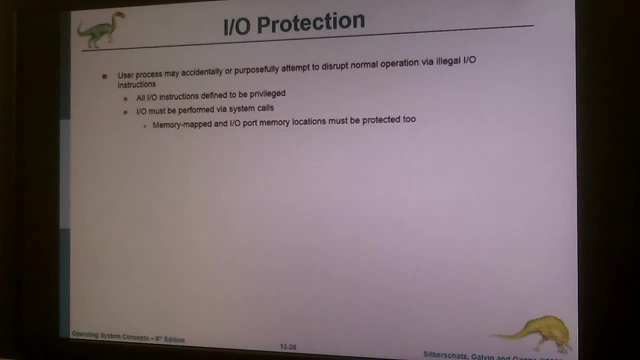 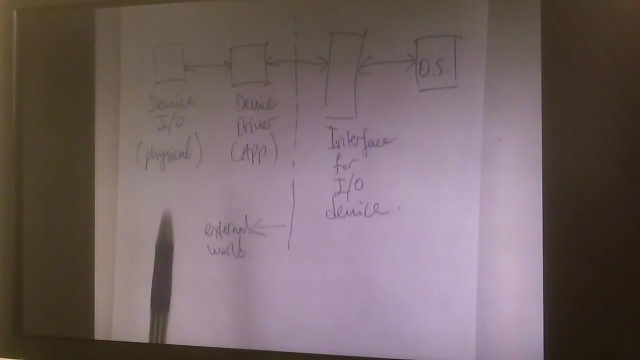 generate an error, right, you have to tell the operating system. hey, there's a problem, I can't read. you know, I can't keep trying this because it's broken now he cannot push sometimes you have to stop, all right, so that's, those errors has to be handled by who? okay, that's a real good question in which box I should. 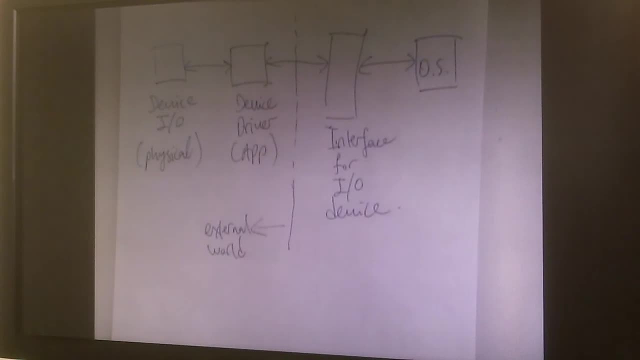 generate the error. I had. the device, this is the physical thing. I mean, this is the printer, this is the hard drive, this is the CD, whatever. and this is actually the source of the error. right, this is the mechanical or electrical or whatever kind. I have an error, I can't do what I'm supposed to do and that device is not responding. so 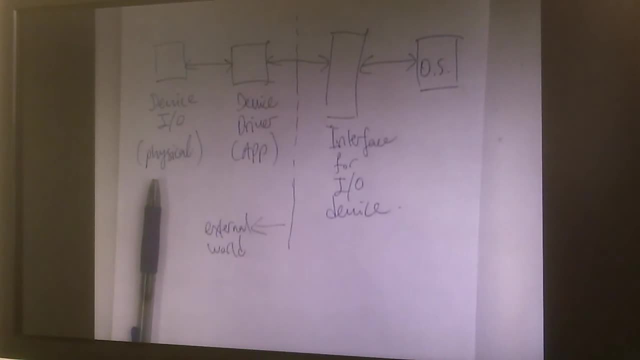 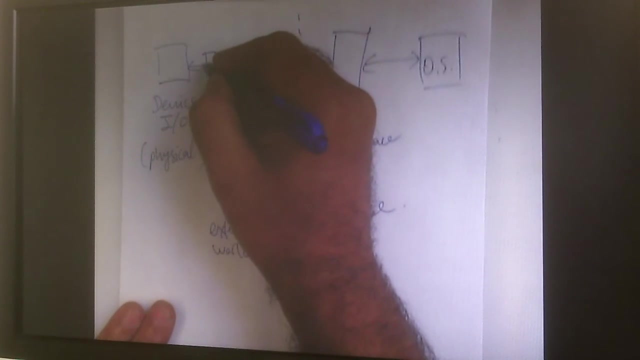 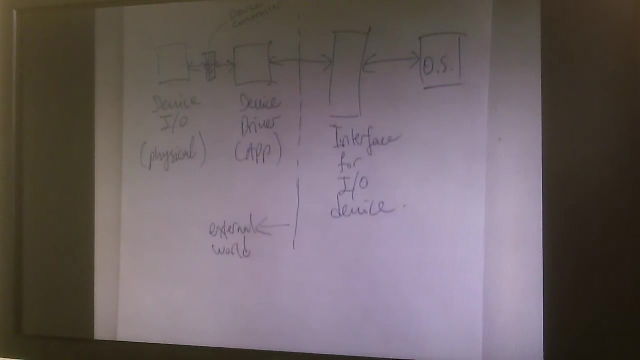 this is a bunch of you know electric parts and mechanics. it cannot talk to me, cannot give me anything, it doesn't have a software or whatever, but this. well, we forgot something here, by the way. what is this thing? device controller? this is the you know PCB, that the green thing anyways. and 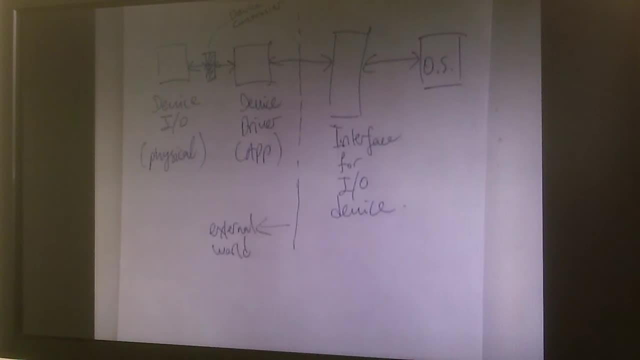 device controller is also a bunch of electronics- cannot talk to the operating system. well, it's some, in some ways it can, but it cannot really report an error, right? what do you think? should I go for the driver application- I'm sorry, the device driver- or should I go for the controller? which one? or the operating system itself? 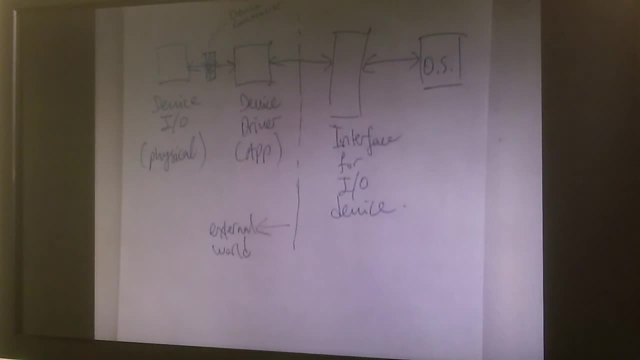 who is generating the error and who is handling the error. well, the device is generating the error itself right there, physical, whatever, or electronics, some some sort of problem. this is the air source out there and actually device controller is sending out some signals to the device driver because right, device driver understands the language of the controller. that's. 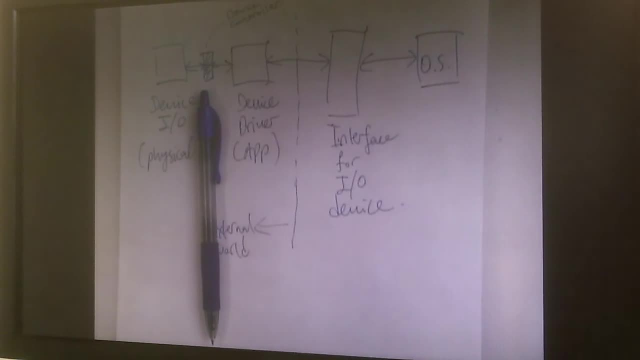 the only thing that understands the device controller's language right, and also a device. there I was capable to talk to each other on the go because it kind of west side what seems to into the operating systems interface. so this guy is the most important one for me, even though the device controller tells me, hey, there's an error here. I 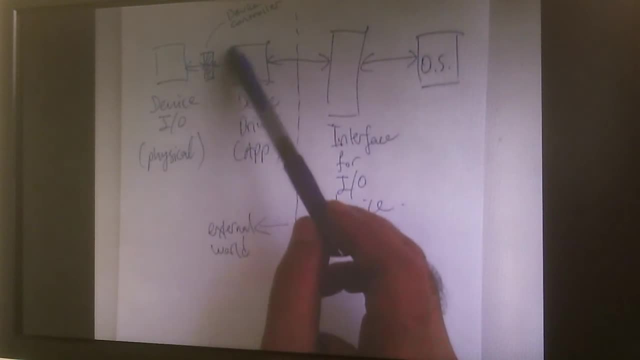 can't. I have a bad block here on the hard drive. even that controller tells that the reporting person is a device driver. that is the piece of application, piece of software sends the required information to the operating system and operating system takes care of it right and in most situations. 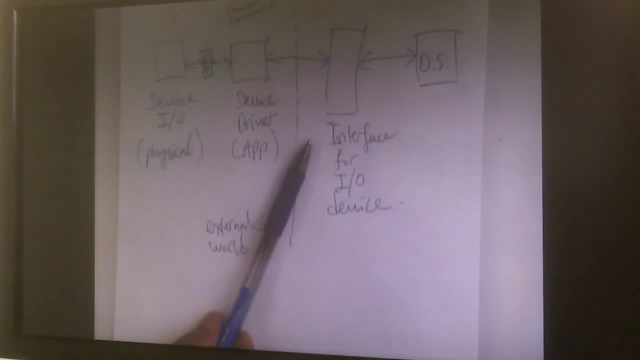 the controller or the device driver will have some sort of trap to recover from the error. in the old days, for example, we had this application, external application- to search through the hard drive and mark the bad sectors on it, right, so you don't want to use it again. 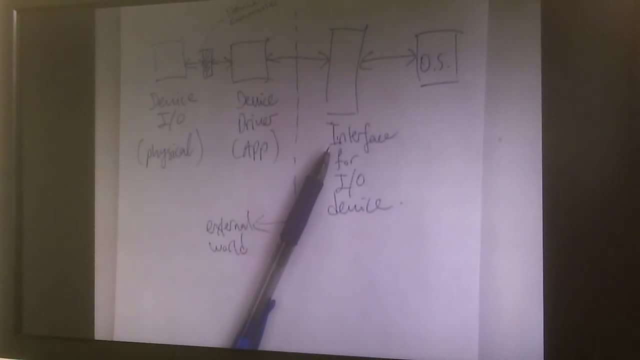 and lose your data, that we were using an external application for that. but in the latest hard drives right now it is embedded into the controller. all right, that PCB at the back of the hard drive it has a list, a flash drive which holds a list of the bad sectors in it. all right, so it never, ever touches that bad. 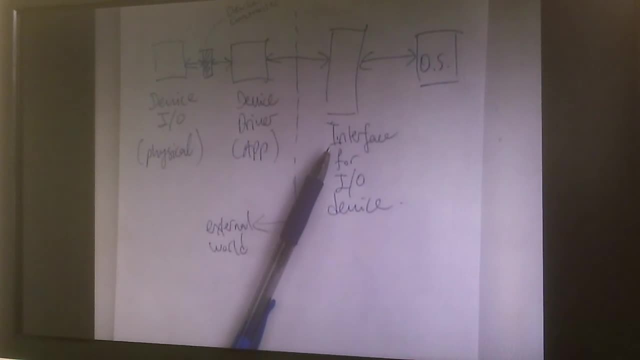 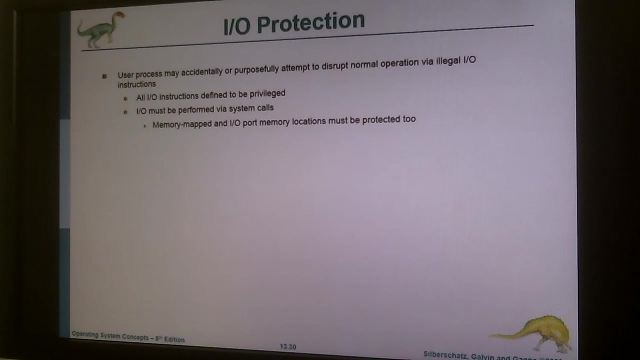 sector, so you will not face any problems later on. okay, so let's go back and finish this up and then quickly go through the chapters, all chapters, and I'll tell you which one is important. we're approaching to the end of the class, so system called kernel data structures. 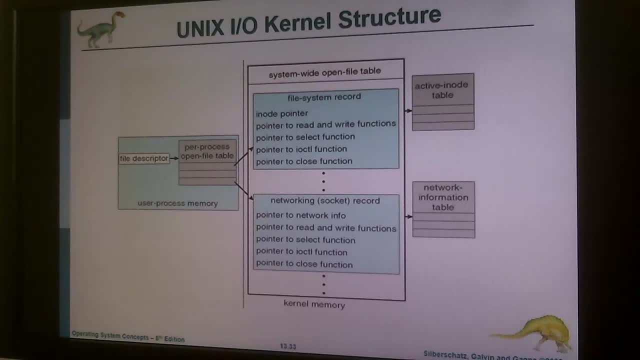 and the moral of this story all about. you know the data structures are built in the kernel Channel, data structures for each specific io device. as you, no it knows. we have the interfaces for each type of I devices in the or Kernel IO sub system and according to the type or I a device, we also have data. 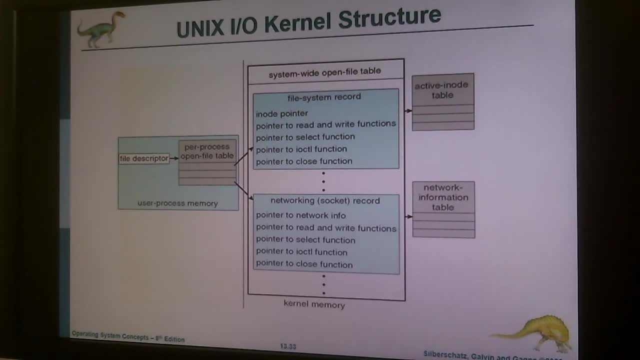 structures built in in the LS. In this analogy, e- стор Credit, Absolutely free to interface for each IO device type and it's going to be faster to communicate with those. For example, if you're talking about a file, it's an IO right. 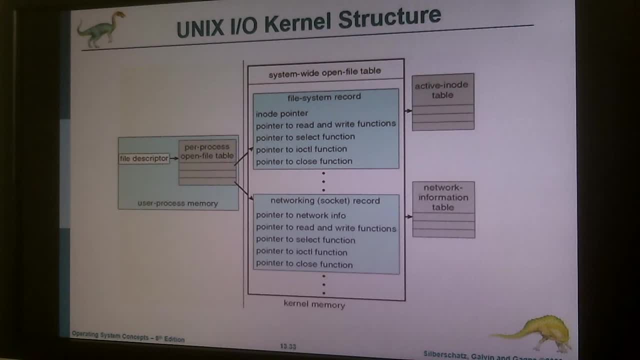 It's an IO device. You know a file could be in a hard drive, in a CD, in a flash memory stick et cetera, But at the end it is a file right. You have a structure for a file and you have a system. call for it. 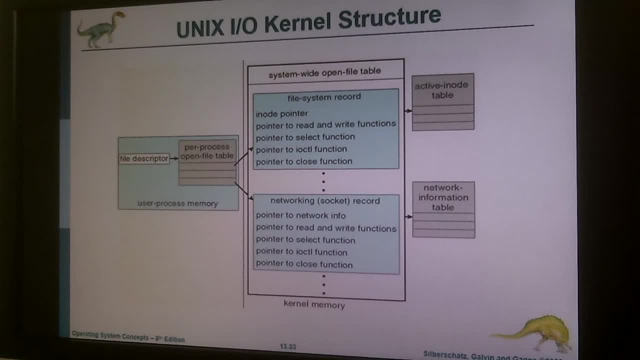 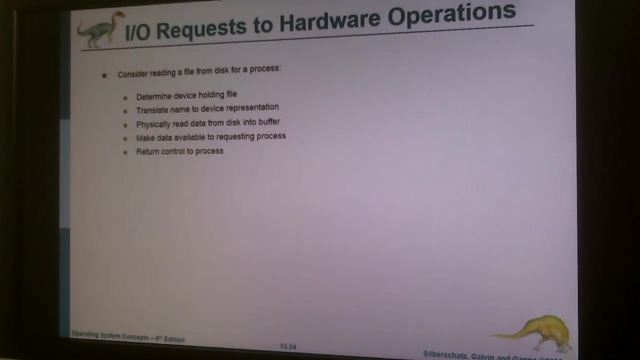 In your language, for example, programming language, you have methods, functions that cause those system calls at the background, So it will actually utilize those data structures built in in the kernel. We're just saying that, hey, there's something like that and use it, you know. 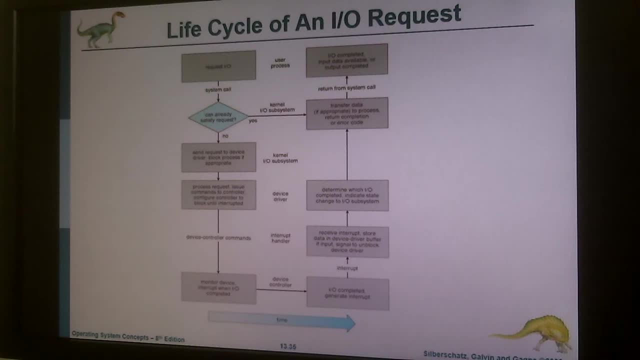 All right, It's a flowchart. Owen And IO request flowcharts are used for algorithm design in your programming. Maybe you saw them, You know: start yes or no, generate if-then-else structure with diamonds, et cetera. UML 2.0.. 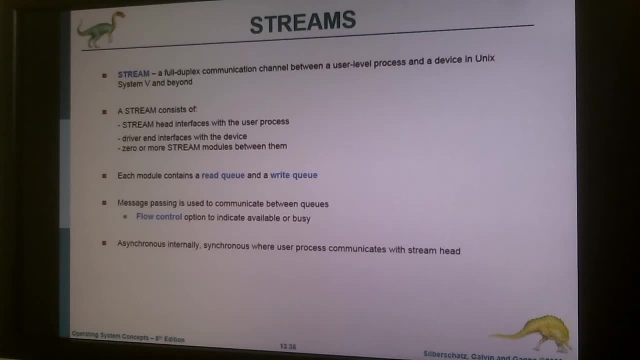 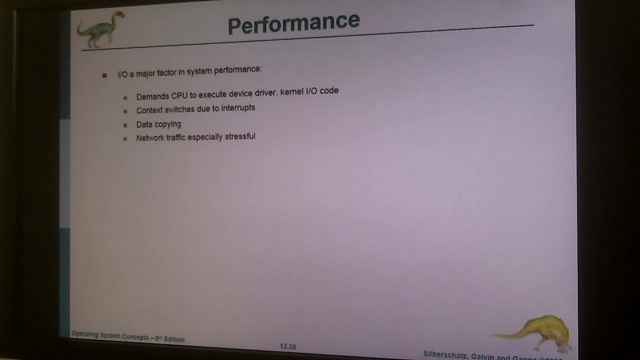 This is something like that. You don't have to worry about this one. We talked about those streams, Let's start with that one. We have the. That's good, Yeah, Yeah, Yeah, All right, properly and accurately. That's what we are trying to do. Sometimes you can keep. 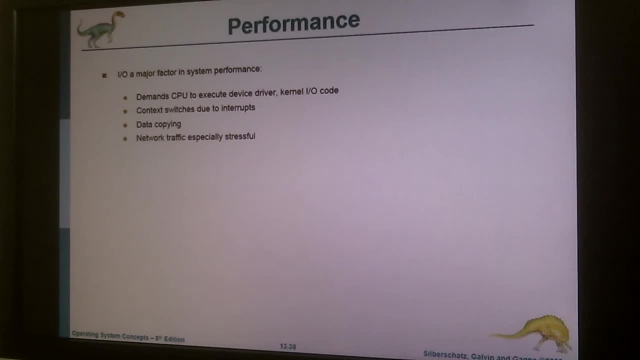 the CPU utilization high, very high. Sometimes your IO will take a lot of time, The CPU will have to wait for a long time, but at the same time IO will do a lot of jobs etc. But overall the operating system design. 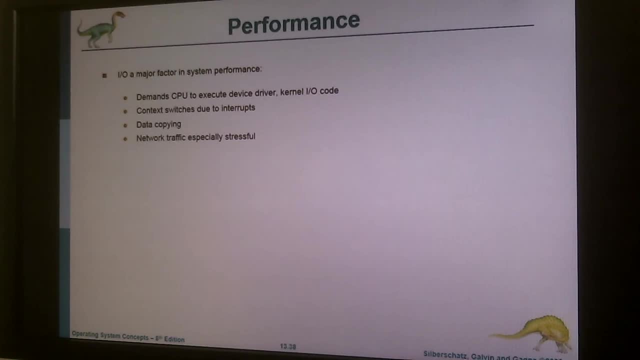 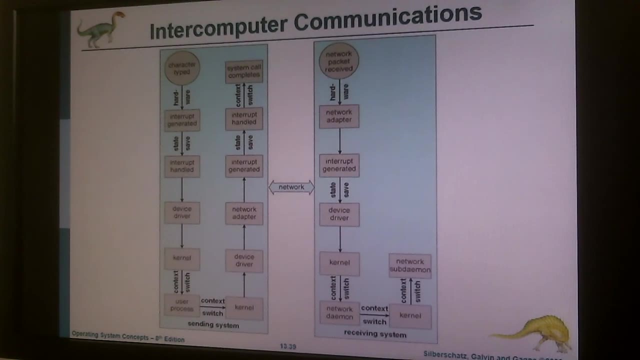 principle tells us that we need to minimize every operation. We have to make everything fast enough, so when there's a load, the overall performance of the operating system will be really actually nominal. This is a long way of saying. this diagram talks about what's going on when 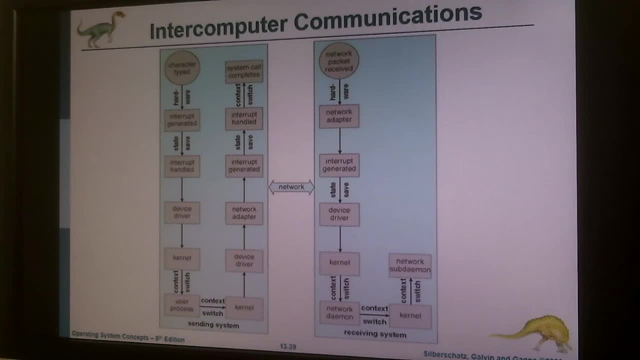 you're trying to do an IO call in the operating system from scratch. On the keyboard, you type a character. After that, what really happens? It's a long way actually, but let's go through. There's your keyboard: You print on a character and then there's an. 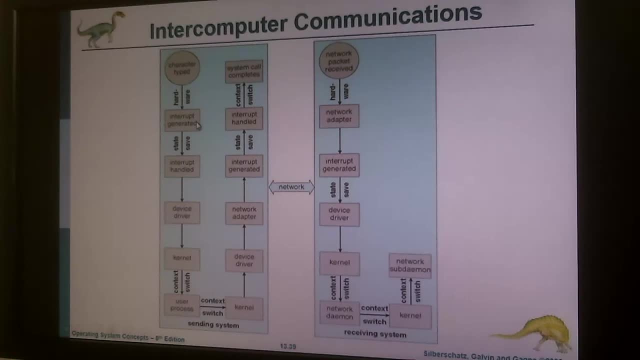 interrupt generated by the keyboard saying: hey, someone printed on something. Or when you move your mouse, hey, someone is moving something. Maybe the user is trying to say something. The user is trying to do something. What should I do now? Take care of the user- Customer is always right anyways- And then your. 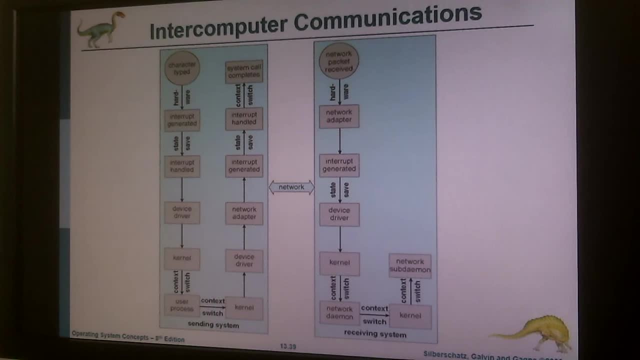 interrupt will be handled by the operating system, But first it's going to go through the driver. right, The device driver And the kernel will take care of the system calls because it's an IO device. Using the interface, it will run the device driver methods. And then, finally, what are we? 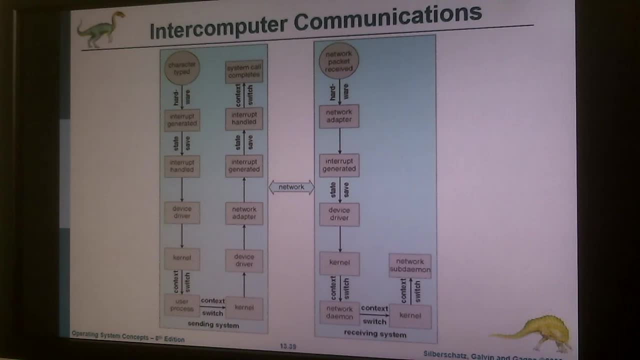 actually going to do is it's going to create the processoh. by the way, this is actually between the remote computers. You know, you type something on the terminal, It shows up on the other side. What really happens here? This is talking. 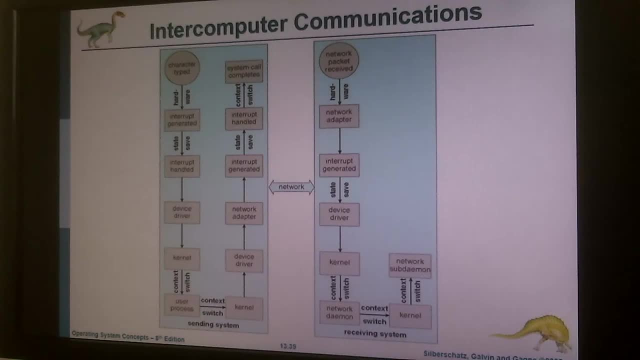 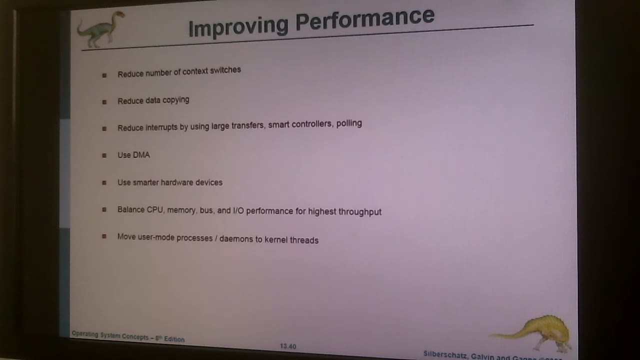 about that. It's not only the generic IO device messaging or the workflow, It is also about the remote IO device messaging. Let's forget about that. The same thing, doubled on the address line, but one side is server, one side is clients. by the way, it's a little bit. 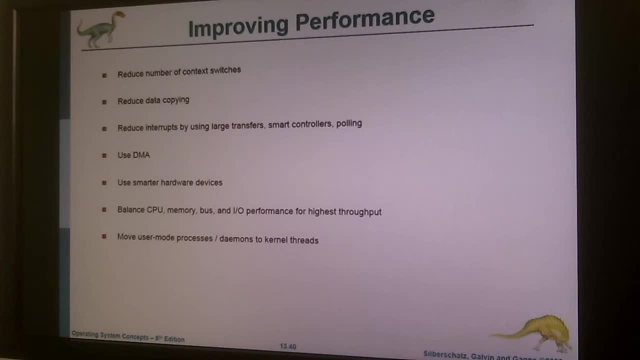 different. I mean, what can you do to improve your IO device management performance? you can reduce the number of. you should actually reduce the number of context switches. you remember what was it context switch? come on, you can do it. it sounds familiar. okay, it's a part of CPU scheduling. 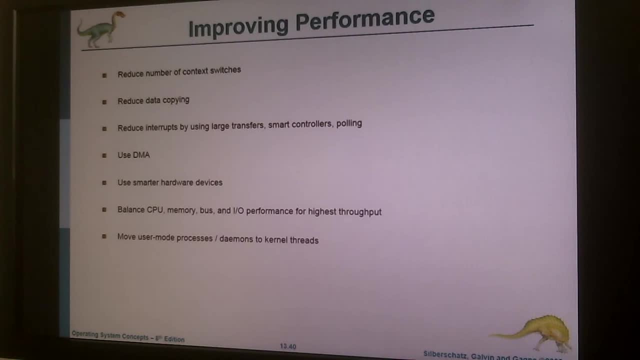 all right. what do you do when you put a process into a waiting queue? or after putting a process into a waiting queue, what do you do? you switch to another process. that is context switch. so if you reduce the number of context switches, that means you're saving a lot of- you know, CPU cycles, while you- someone I was- 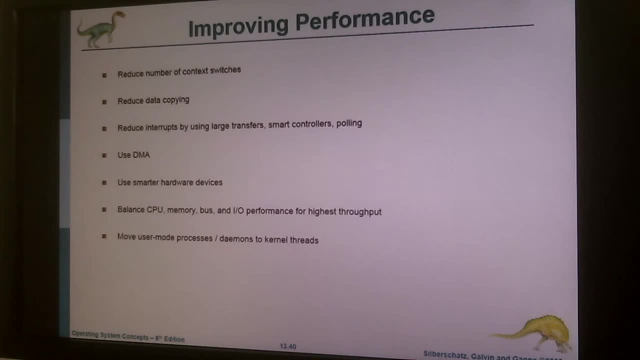 asking about BIOS programming here. he was you right. yeah, and I was saying that if you, you know, as a device driver, developer, you can find, you know you can find a good job. they will pay you a lot of money because not many people are writing twice drivers. if you ride your dry and dry Jah sr yourself in that. 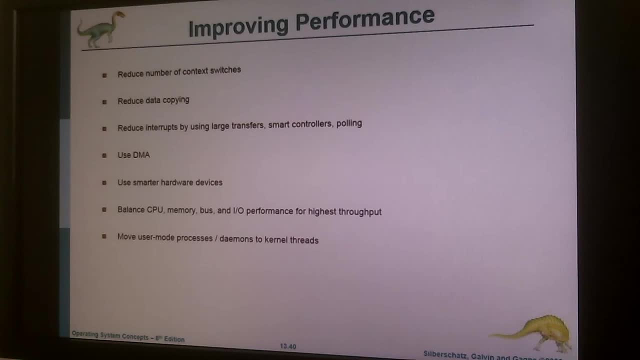 great, or if you're still, you know- professional programmer, you should try to reduce your number, the number of the contact switches in your twice driver. okay, that means you're going to use thread. that means we're going to use. you're going to handle your ide wise, properly, which will not cause your 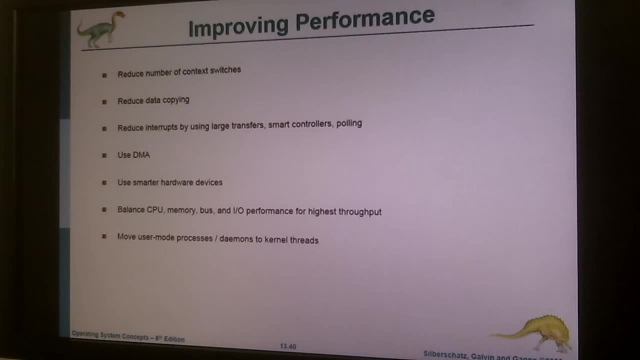 process to be put in a wait. queueksam lists- all right, that's what it means: reduce a data copying. instead of copying, just move it. try to move it and data copying actually is a problem. when you're copying a lot of data, you know when you're moving or copying large amount of. 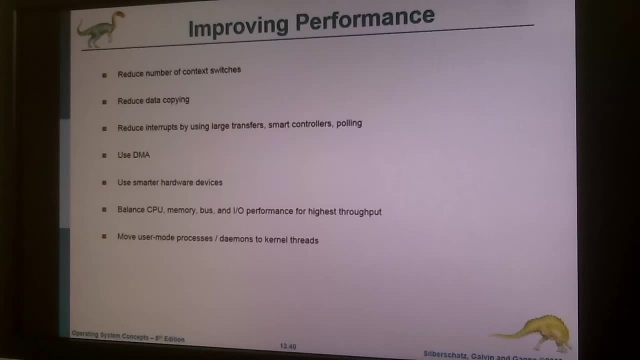 data, it's a problem. so if you want to do it, if you had to do it, do it efficiently in a way. reduce interrupts by using large transfer, smart controllers, polling, use other technique techniques or algorithms to reduce interrupt number of interrupts in a unit time. use DMA, it says, and mapped memories instead of. 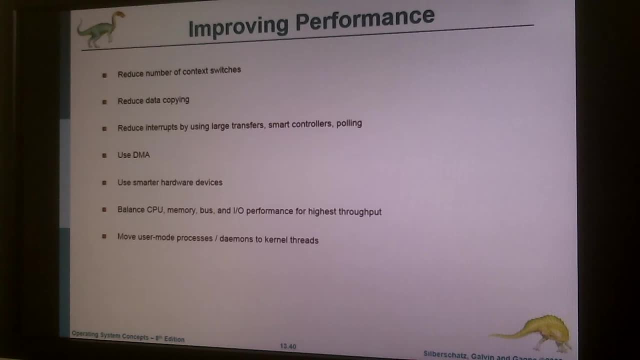 using the CPU all the time. use the DMA controller if it is possible, but, as I said, using the DMA accessibility we will generate a lot of security problems. all right, use smarter hardware devices. what does it mean? what do you think it means? use smarter hardware devices to improve IO device performance. what does it mean? what could? what it? 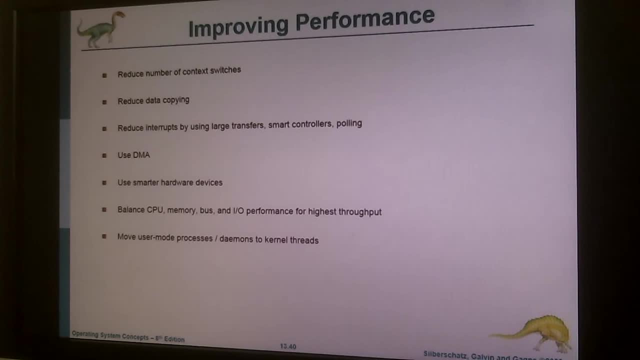 could be possibly about being smart or dumb. as a hardware- macOS, macOS, Android, MacOS, MacOS, MacOS, MacOS, MacOS, MacOS, MacOS- And its SSD part is only 8 gigabytes, but the other part is terabytes. It is called a smart hard drive, but if you have a magnetic drive only, let's call this dump drive. 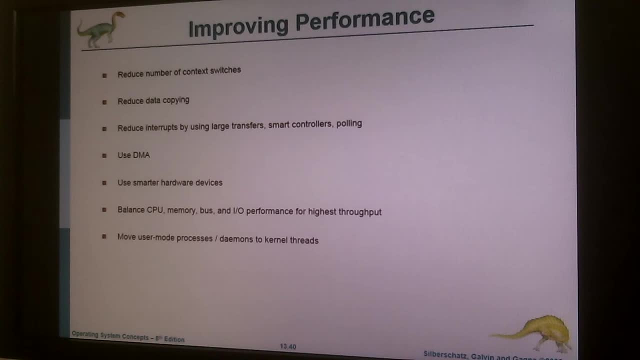 What do you think? why we're calling the other one smart. Not only that, how it's possible to make it. you know how can you make a hard drive faster with an SSD or some other technologies? Well, you're actually using statistics, algorithms, selective data processing. let's say: 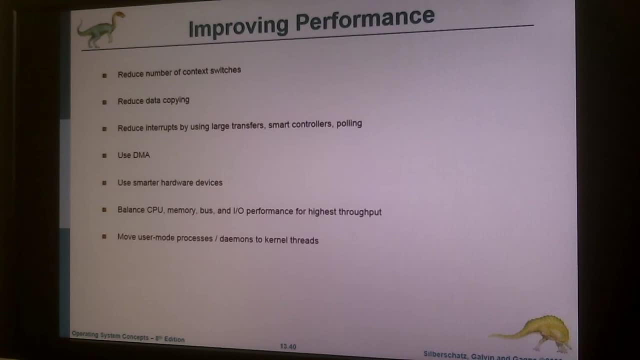 What happens with the SSD hybrid. You know, as a user, you're using some files right In your hard drive. after a while, let's say two hours later, your hard drive makes a table for each file, says: you know, this file is reached. read two times. 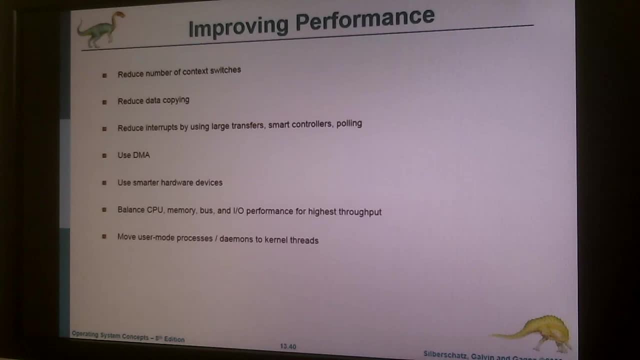 This file is read ten times. This file is read one time. This file is read never. It was not read at all. And this one was read and modified, etc. There's this huge table And then, according to that table, it says: you know, statistically, the user will probably use this file in the next two hours too. 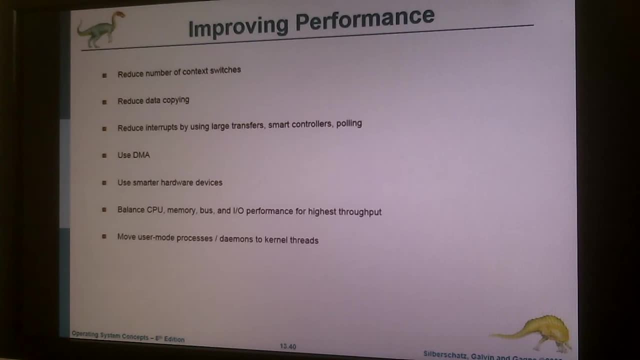 So you know what? Let's move this file to the SSD part of the drive, And SSD part is faster than the, you know, magnetic disk, And the next time you reach that file it's going to be way faster. So it is not only for the user files, by the way, for the operating system files too. 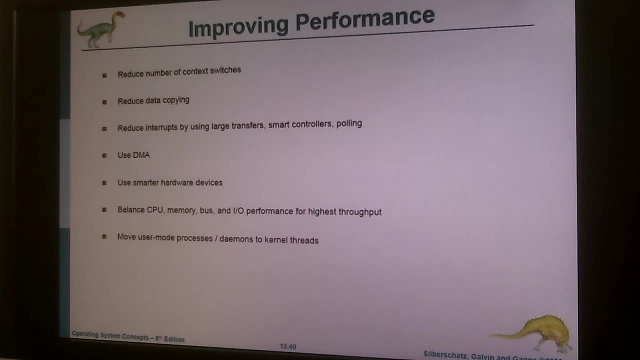 Many of the operating system files are actually read many times right during the operation. you know when it's running, when your computer is running, But for that very reason, actually your operating system has loaded them up. So the memory, the physical memory, already. 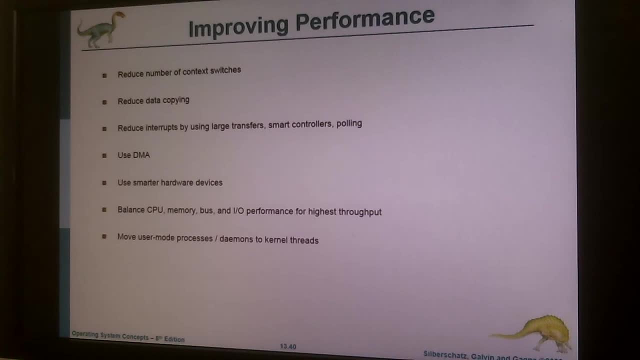 So there's no need to read them multiple times, right? It will just read it once. when you boot up your computer, put everything on the memory right, And then the other files will be read, you know, multiple times from the hard drive. 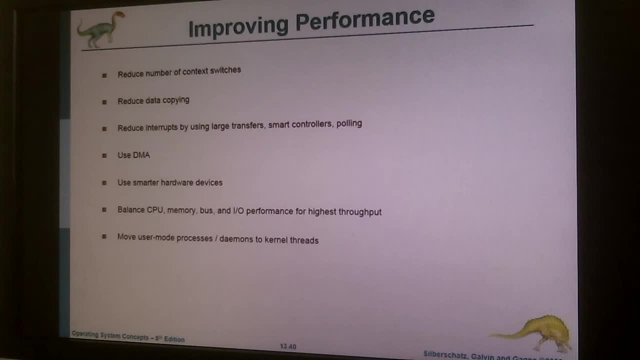 So this drive is smart because it is using algorithms to make the system faster, while it's not really fast. All right, It's making this virtual, giving this virtual sense that it is really fast, but it's not really, you know. 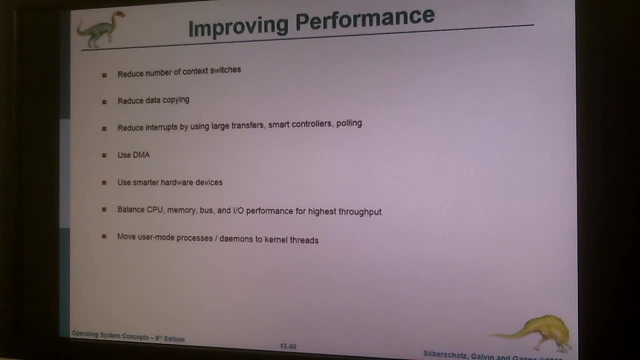 It's just using this 8 gigabytes of fast parts to tell you that, oh, I have a 1.5 terabyte hard drive, which is super fast, But it's just 8 gigabytes, you know, in reality. 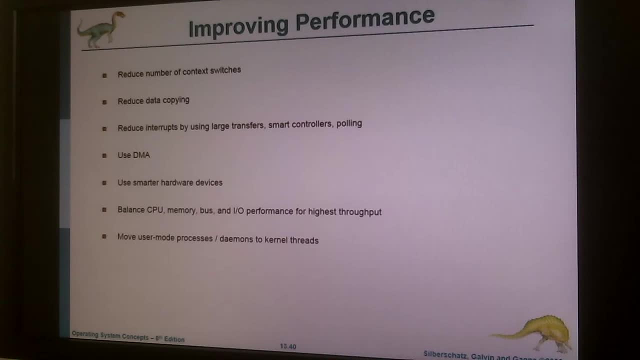 That means you know If you use smarter hardware or devices like this one, your IO performance is going to improve good enough for you and for your company. Balance CPU, memory bus and IO performance for highest throughput. You know the number one purpose of the whole operating system is keep the CPU utilized. 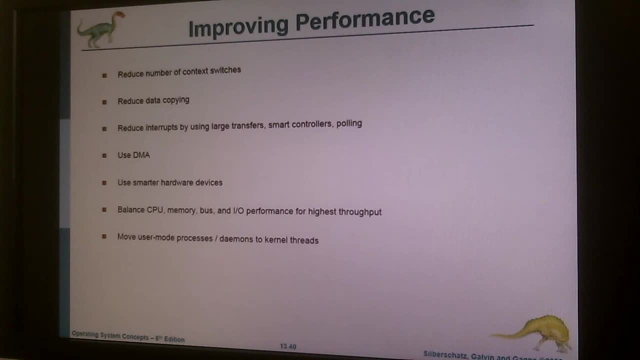 As much as possible You can use the memory efficiently and use the IO efficiently, so that you know the user will not complain. Operating system itself will not complain about speed or whatever, And if it's a, you know, mission critical real-time system, it will do the job on time. 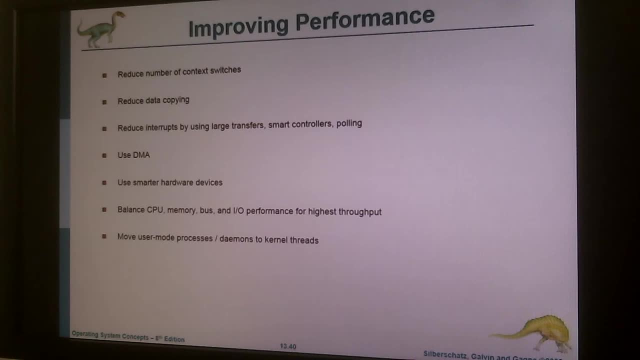 That's the whole idea, the whole purpose. right, Balance everything, Move user mode process, Adjust daemons to kernel threads- All right, If it's possible, if you have multi-cores, that is really good for you to use threads. 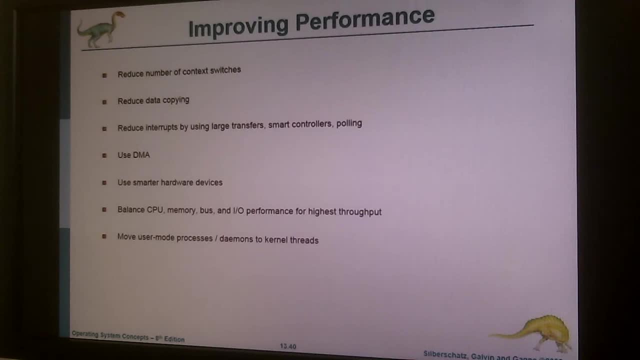 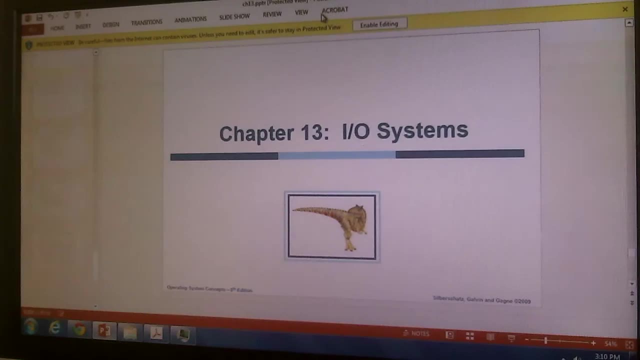 And if you can program your application using threads, you will utilize most of the CPUs. That's what it is. Oh my gosh, It's end of the video. All right, Let's go for, Let's go for, Let's go for. 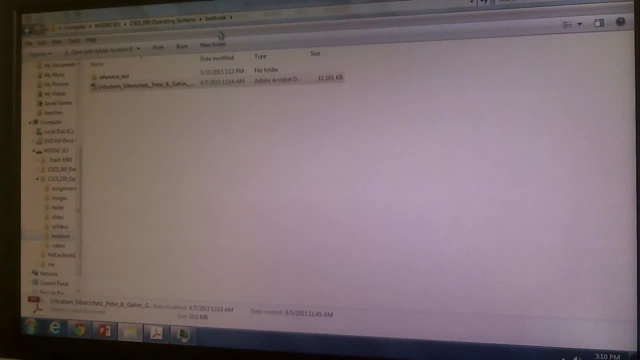 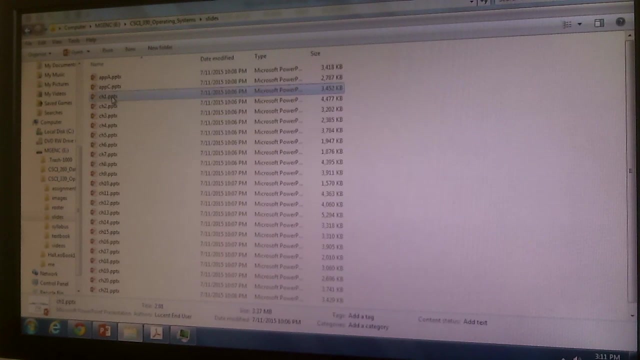